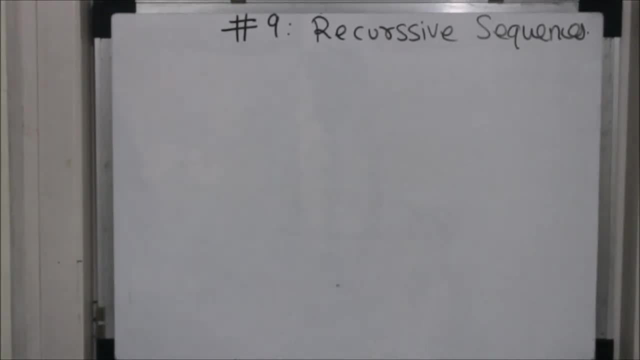 Hello everyone. So today we will talk about recursive sequences. So in the previous lecture we talked about monotone sequence and the bounded sequence And I told you why do we need them. The reason was because we have a theorem that if a sequence is a convergent, 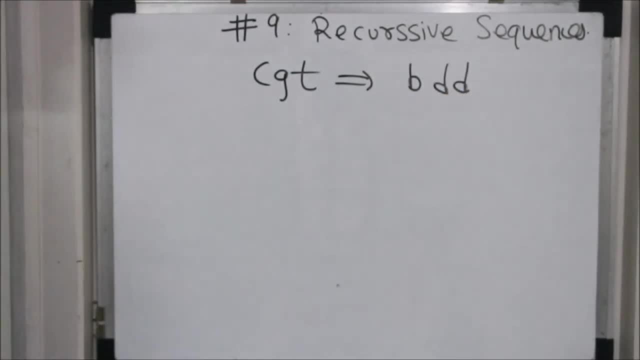 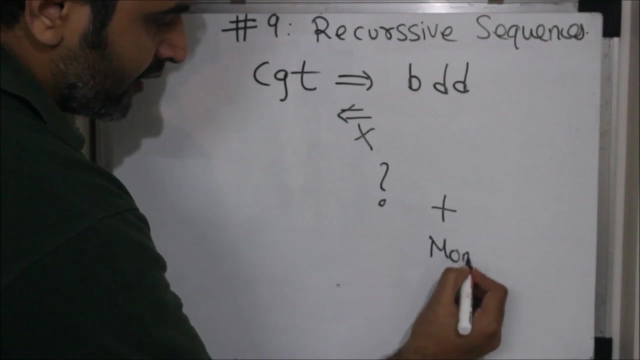 sequence, then it is a bounded sequence And the question is: is the converse true? And we saw that the converse is not true. So therefore the question arises: when will be the converse true? So that was the question. So the answer was: if the sequence is bounded plus monotone. 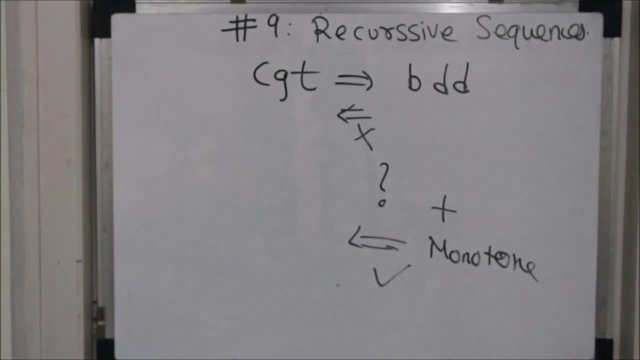 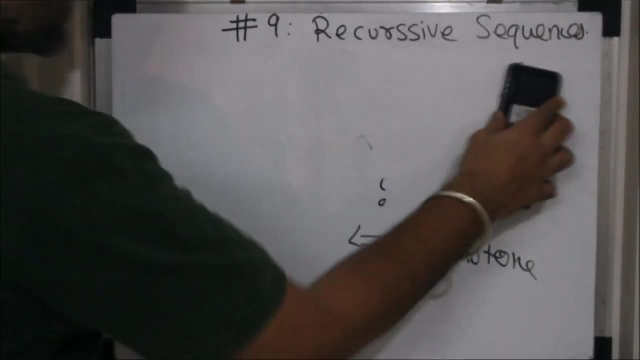 then the converse is true. So this is what the statement we saw in the last session. So today we will see what are recursive sequences and how this theorem helps us to prove the convergence of a recursive sequence. So what is a recursive sequence? So recursive sequences. 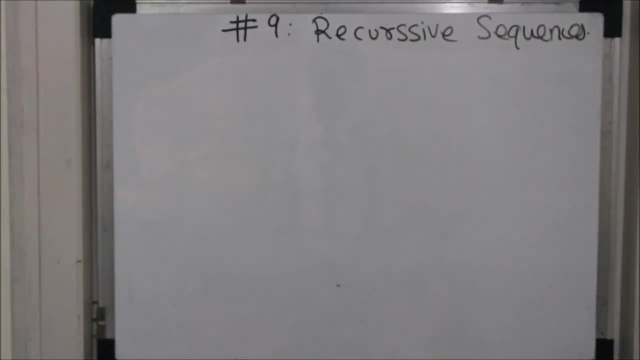 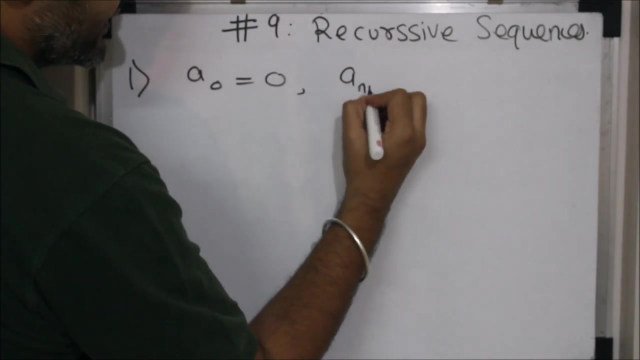 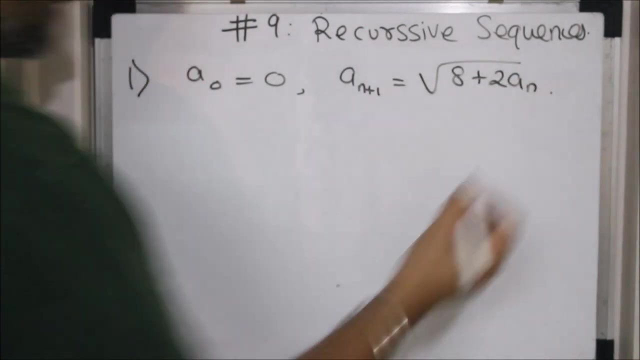 are nothing, but Usually some value will be given to you. So let me take an example directly. So suppose, if I give you, the first term is zero and the next term is depending on the previous term with some relation. So this is the relation which I have. That means what my first term? 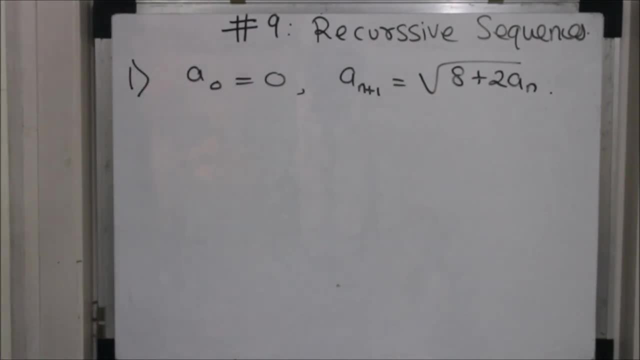 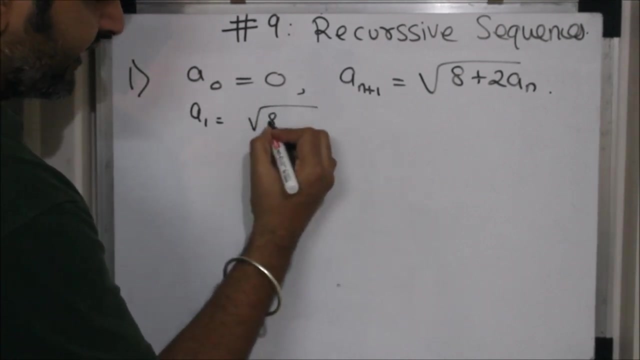 is zero and second term is not given you directly but they have given you some relation. So this is called as a. So if you want to find the next term, you have to use this relation. So this is called as a recurrence relation. So what will be a1. If I put n equal to zero, a1 will be root of a plus 2. a naught, because 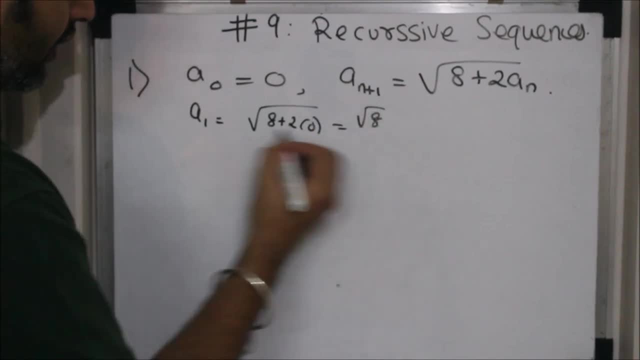 my n is zero, So this is nothing but rooted. What will be my a2. a2 will be? you put n equal to 1.. So 8 plus 2, a1. 8 plus 2, what is a1. Rooted? And this way you can find all the. 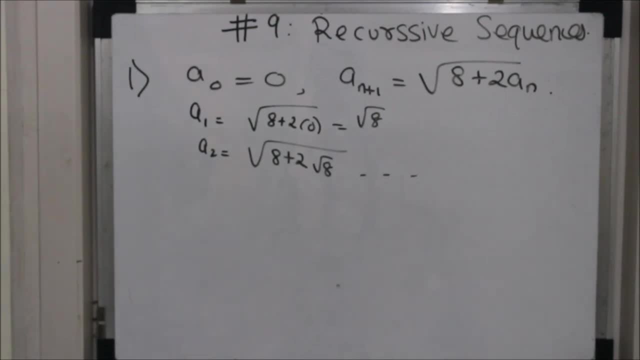 terms of the sequence. But then now, if I want to check whether this sequence is convergent or divergent- It's difficult to check- I can't apply my theorems which we saw previously. Previously we saw sandwich theorem, We saw continuity theorem, We saw L'Hospital rule. So we can't use those theorems over here because 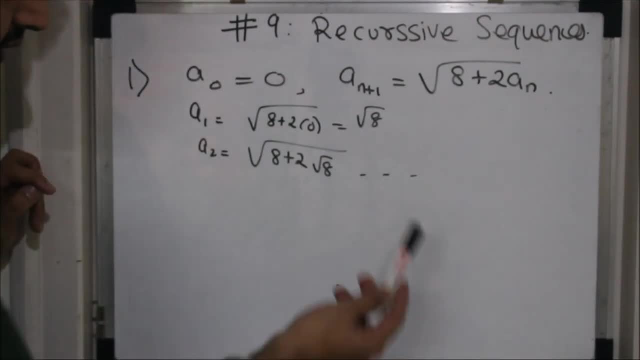 there the nth term was depending on n, Whereas here the nth term depends on the previous term. So it's difficult to apply that theorem over here. So what we will do is we will use the statement which I just now stated. What we will do is we will show that this sequence: 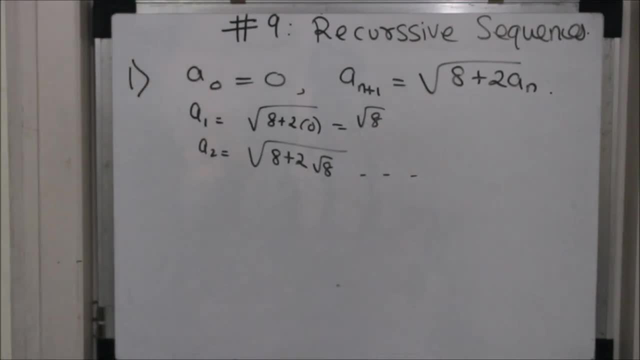 is bounded and this sequence is monotone. And once you prove that your sequence is satisfying these two condition, So by monotone bounded theorem what we can conclude that this is a convergent sequence. So now to prove such thing, there is no one proper way that, ok, you have to go by this way and you will get the 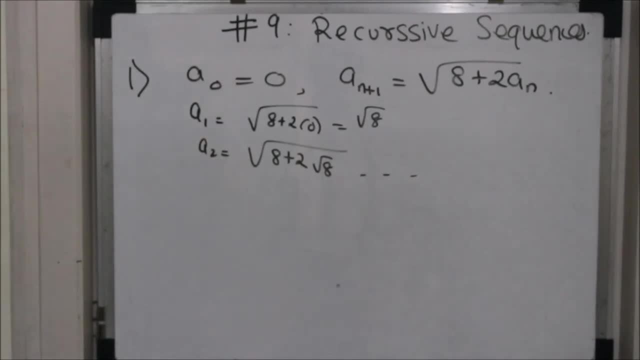 answer. So I will take some three, four examples so as to get an idea on how to prove such kind of things. So let's continue with the same example. So I want to prove that it is monotone and it is bounded sequence. So let's see whether this is a monotone sequence or 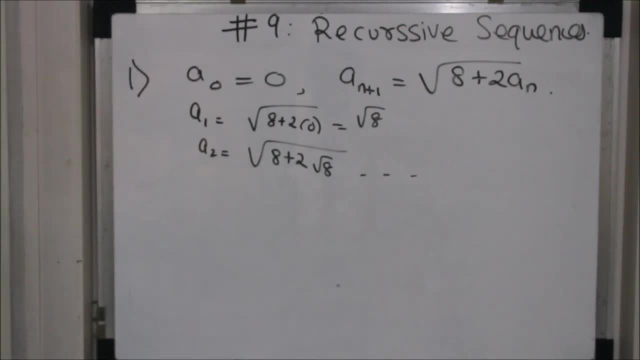 not so from here. so whenever you have a recursive sequence, always write down first few initial terms to get some idea. so here the first term is 0, second term is root 8, then the next term is root of 8 plus 2 root 8, and so on. so from here one can see that your sequence is an. 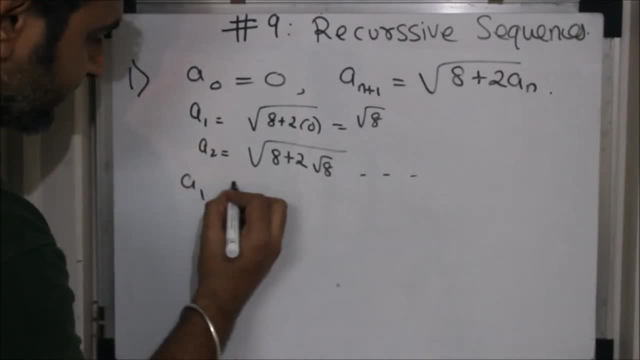 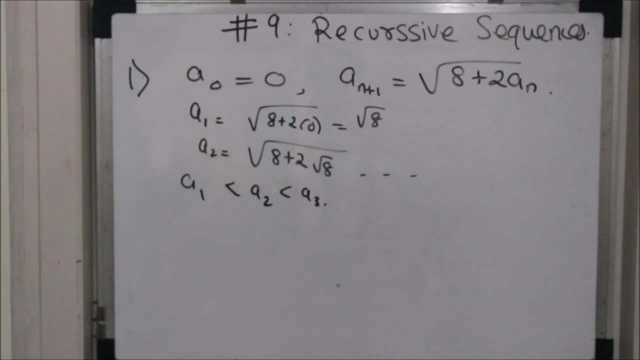 increasing sequence. so from here I can see that my a1 is less than a2 is less than a3, and so on. but then if I want to prove this in general, I need to use a technique which is called as a technique of induction, because I have to prove a statement which is indexed. 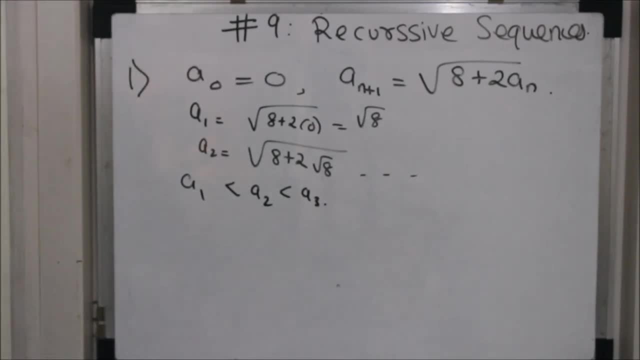 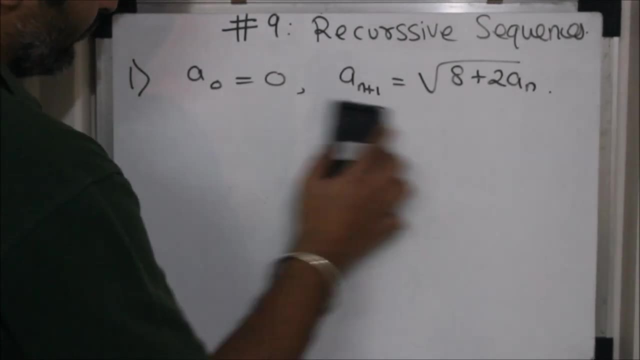 by natural number and whenever a statement is indexed by natural number, induction is one of the best tool you can use to prove your statement. so, in this case, what I want to prove, what I want to prove that the sequence is an increasing sequence. so let your P of. 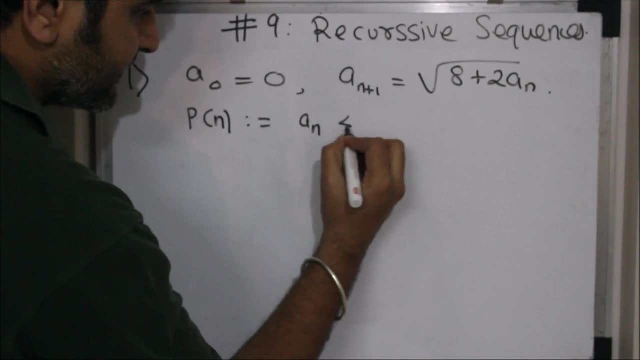 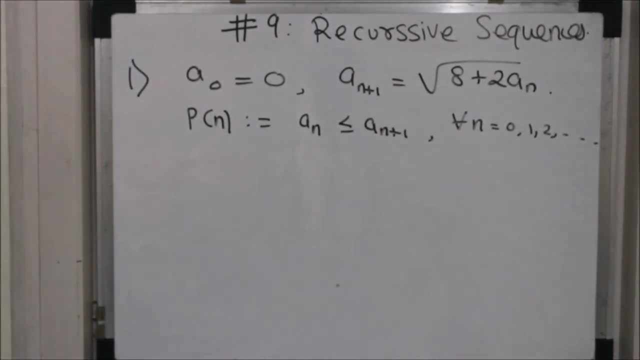 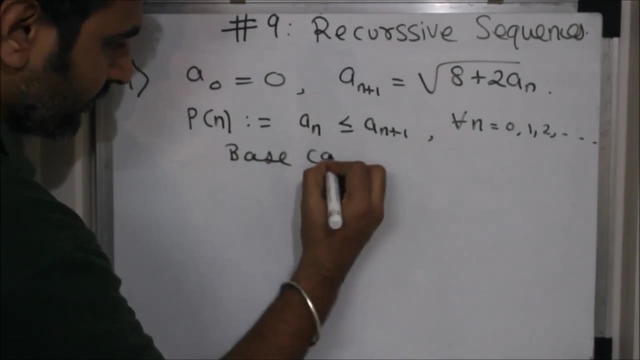 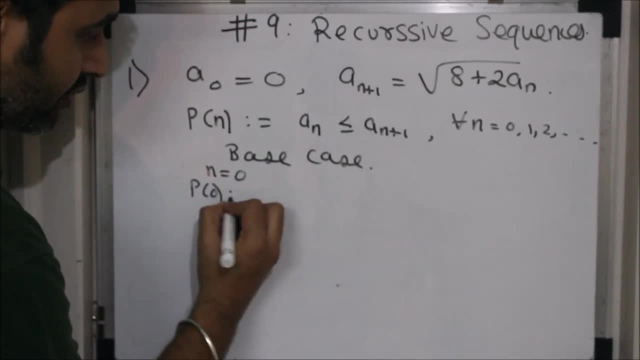 n is 0. that means what is my P of 0? a0 less equal a1. so this is what I want to check, but that we already did right. what is my a0? a0 is 0. what is a1? a1 is root 8, so obviously. 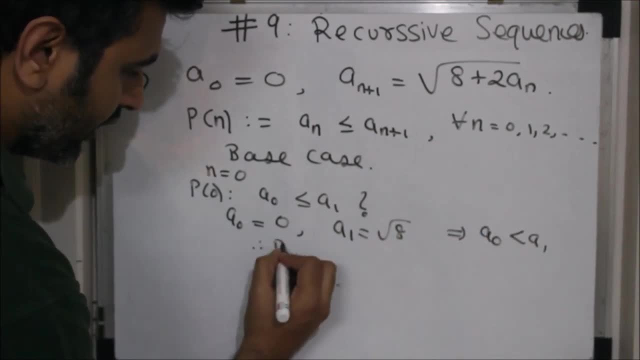 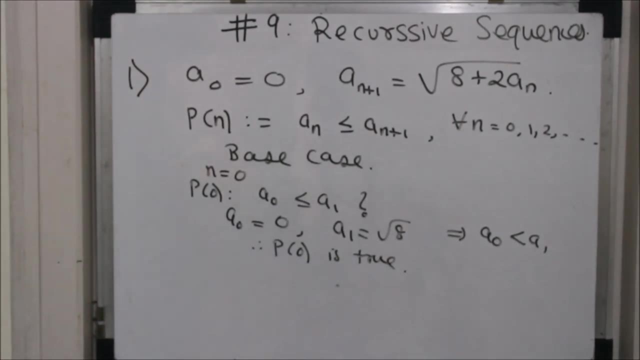 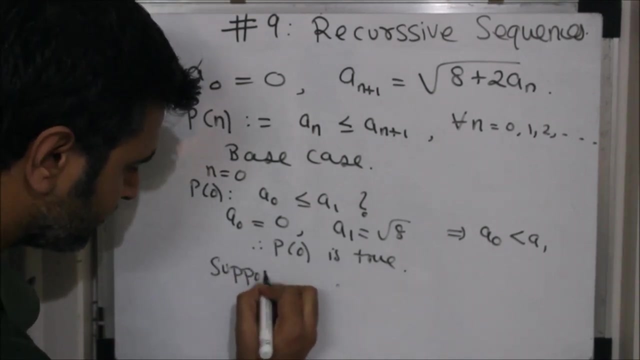 your a0 is less than a2.. less than a1. Therefore your P is true. So therefore your base case is true. Now what you want to prove is: you want to prove the in general case. So suppose P is true. 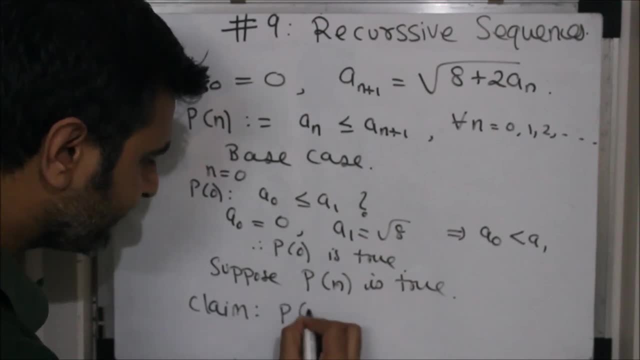 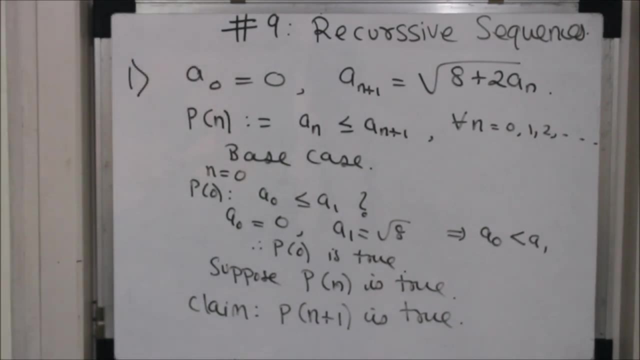 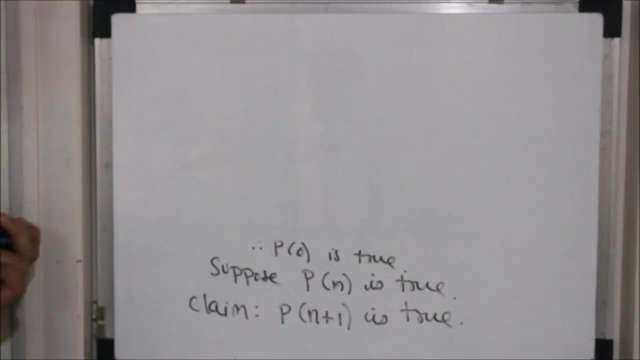 What is your claim? P is true, So this is what you want to prove. Now, P is true means what P is true means what Your P is true. So means what we have, an is less equal an plus 1.. That is what induction hypothesis. and what is your aim? Your aim is to prove: 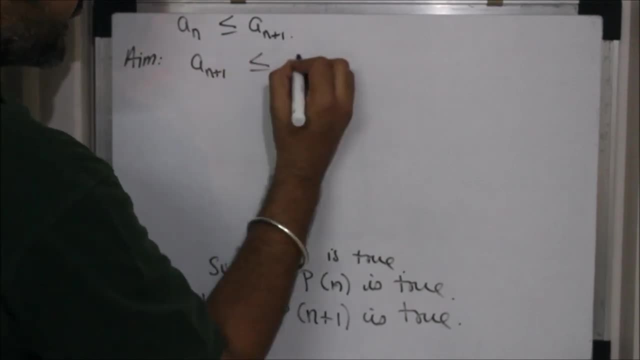 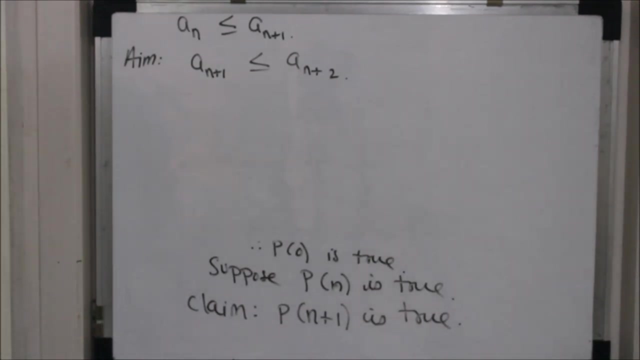 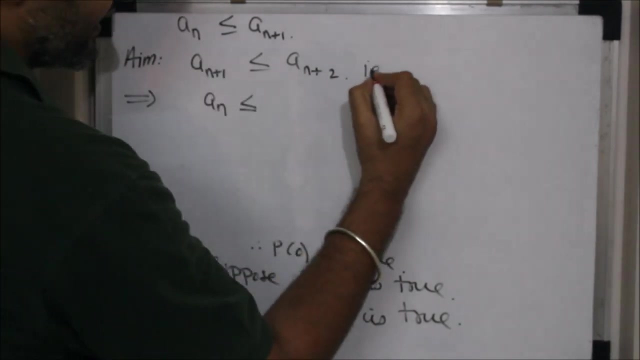 P is true, Means an plus 1.. is less equal? a n plus 2. this is what you want to prove. so in such a situation, we always take the help of the hypothesis and we arrive at our aim. so now, here, what do we have? we have a n less. so what I want to prove here that 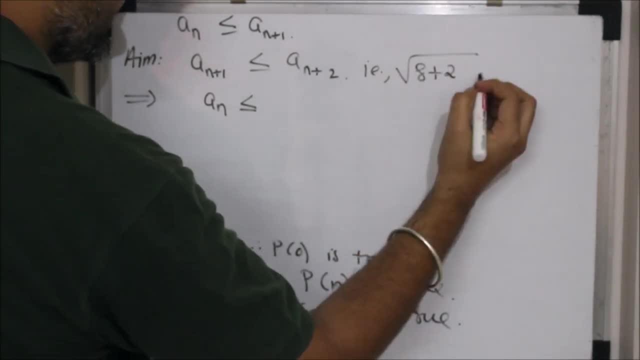 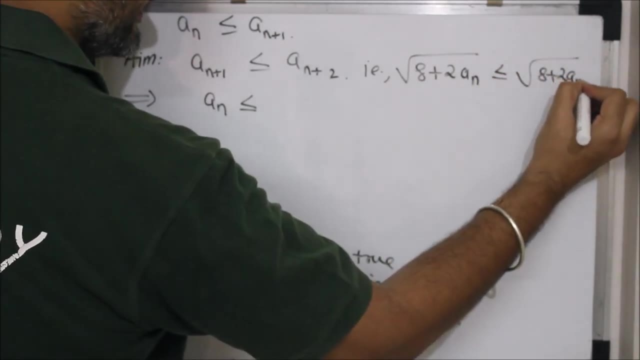 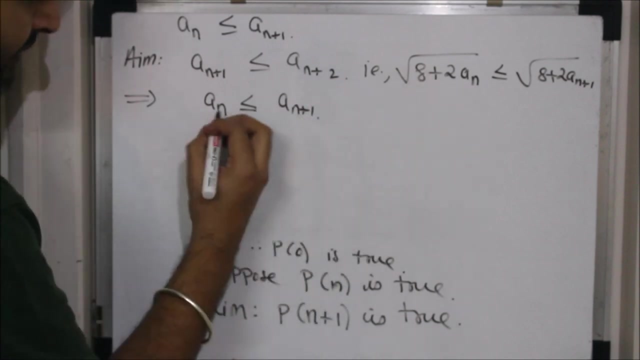 is root of 8 plus twice a n is less equal root of 8 plus twice a n plus 1. so this is what I want to prove. so what do I have? I have a n less equal a n plus 1, so we multiply by 2. so twice a n less equal twice a n plus 1. so I got two. 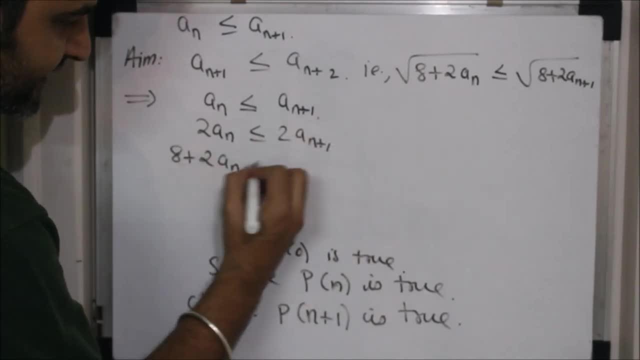 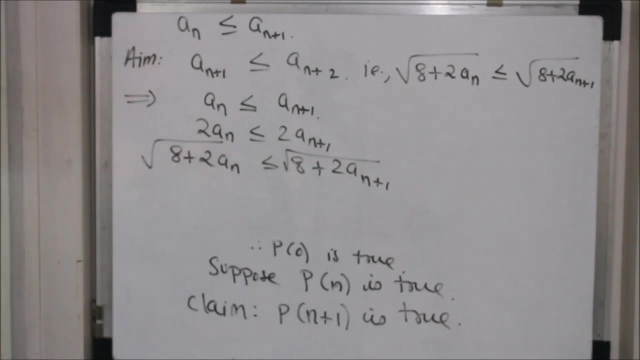 over here. you add 8 on both sides, so this is less equal. 8 plus 2, a, n plus 1. you take square root on both sides. your square root is an increasing function. so therefore, when you apply the square root, your inequality will remain the same and 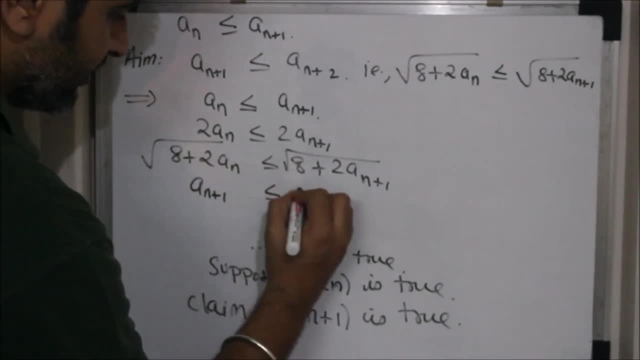 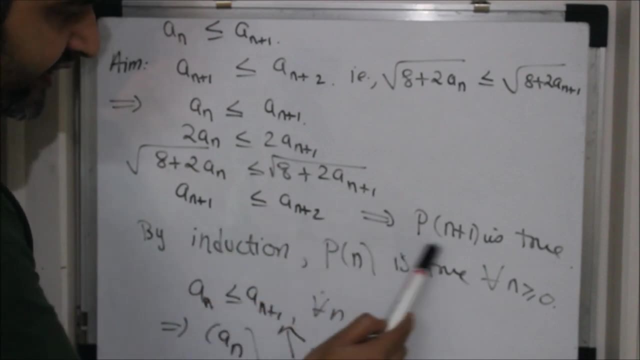 therefore, this is what, this is what a n plus 1, and this is your an plus 2. so what do we get here is an is less equal to an plus 2, so this implies that p of n plus 1 is true. and since p of n plus 1 is true, so by induction we can. 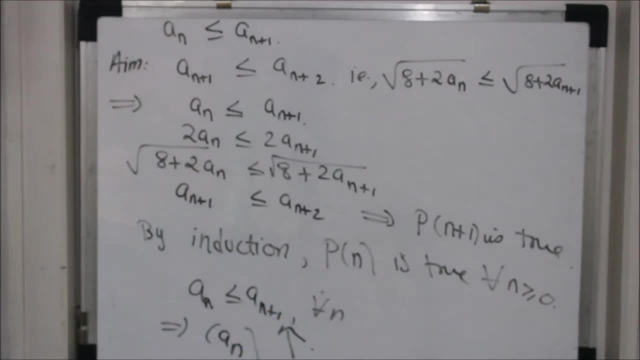 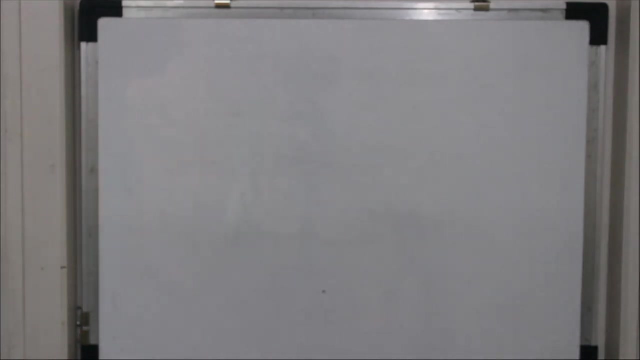 say that the statement is true for all n greater or equal to 0. so what do we get? is our? an is an increasing sequence. that's what we get over here. now we got that an is a monotone sequence. so now to prove convergence, it only remains to show that the sequence is a bounded. 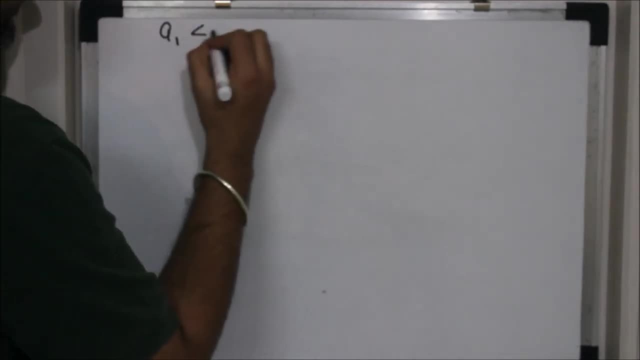 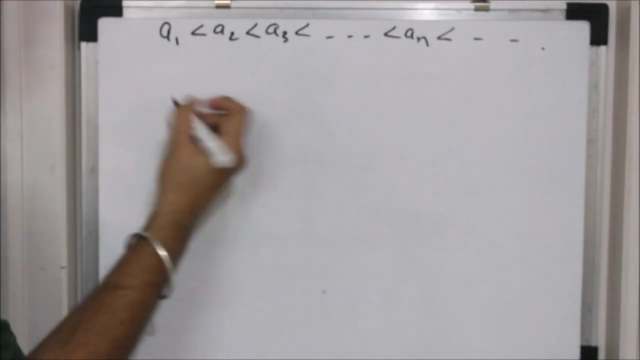 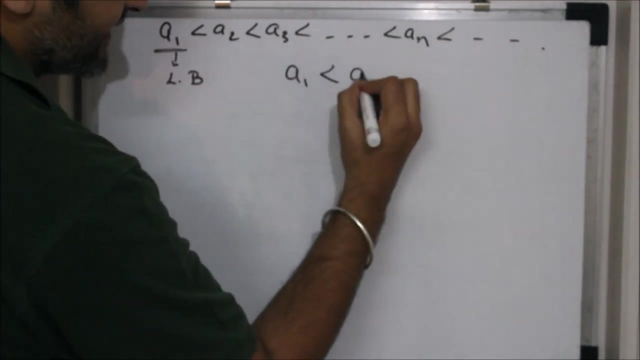 sequence. now, what i know is it's an increasing sequence: a1 less than a2, less than a3. so since it's an increasing sequence, therefore, this a1 will act as a lower bound for the sequence. so that means what i have, a1 is less than an for all n. so i got the lower bound because. 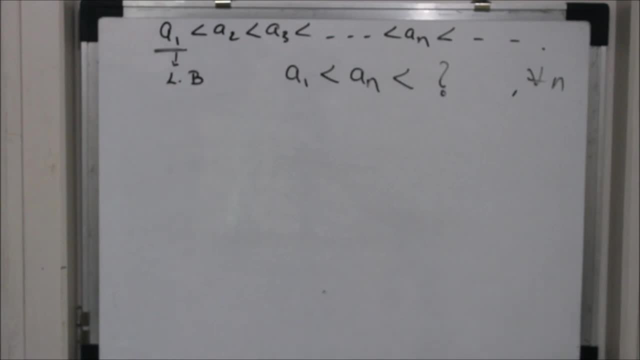 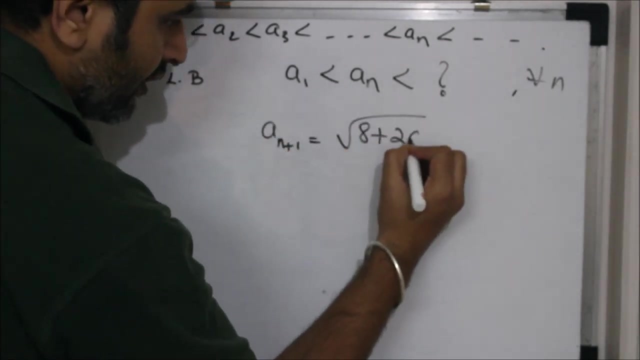 an is an increasing sequence. now question is: what would be my upper bound? so i need to find the upper bound of the sequence. well, it's not that easy to find upper bound of the sequence, so one of the trick is what to do. is you assume that this sequence is a convergent sequence? you assume that this is a convergent. 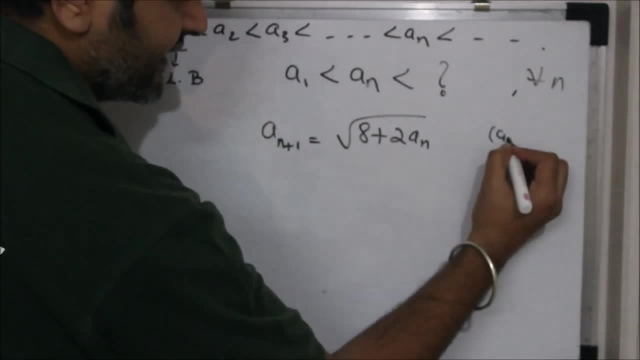 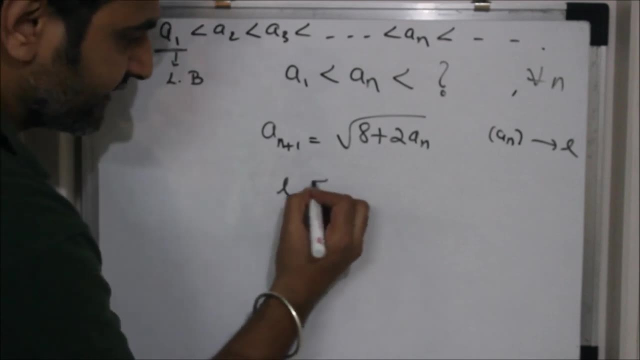 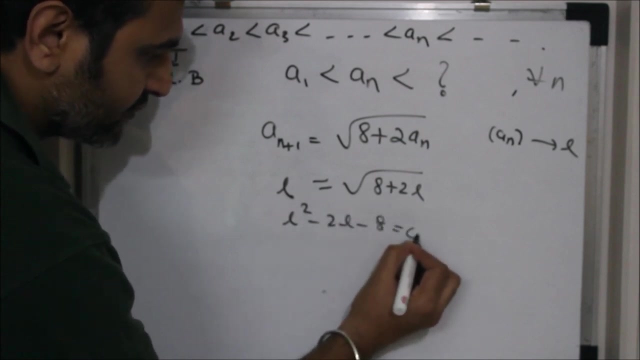 sequence and suppose it converges to. suppose your sequence an converges to l, so your an plus 1 will also converge to l, because it's just, they're the same terms of the sequence. this is what i get is 8 plus 2l. so when a square, l square minus 2l minus 8, equal to 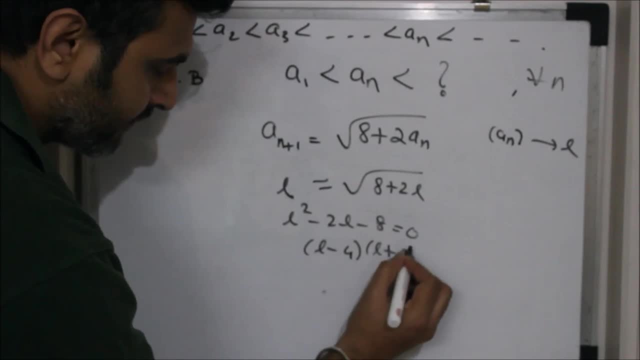 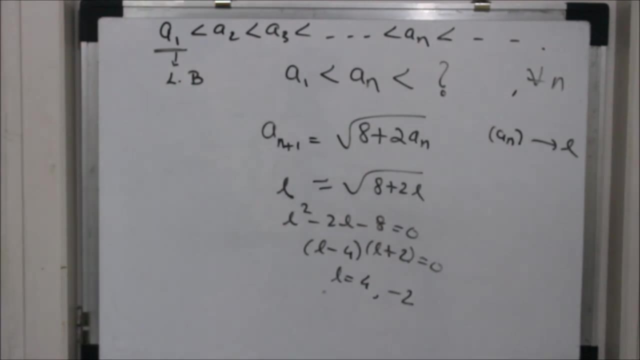 4. what i get is l minus 4, so l equal to 4 or minus 2. but since my sequence consists of positive numbers, therefore the limit also has to be positive. one needs to prove that, but you can assume that fact that the sequence of positive numbers will always converge to. 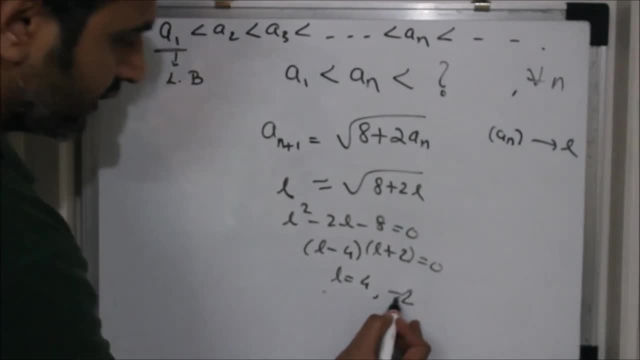 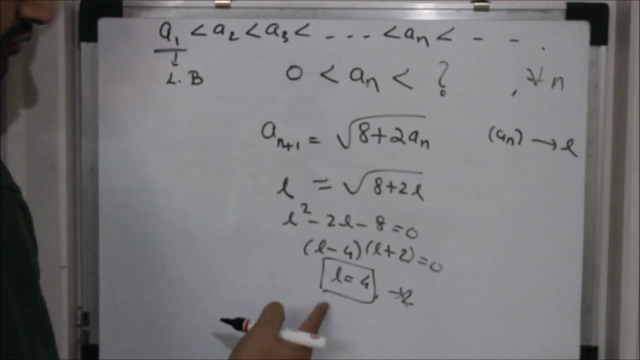 a non-negative number. so here your l cannot be negative. therefore, its sequence is converging to 4, so i know that the lower term is 0, a1 is 0, so an increasing sequence is a convergent sequence and since the limit is 4, what you need to show that now that 4 will act as upper, 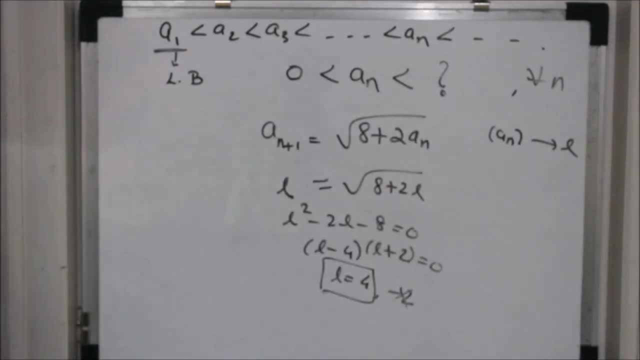 bound. so once i show that this 4 is an upper bound, my job is over. so from here, using this trick, we are finding the upper bound, and once you find it, we need to prove it that all the terms are less equal 4. so now let's prove this fact. so let's prove this fact that your 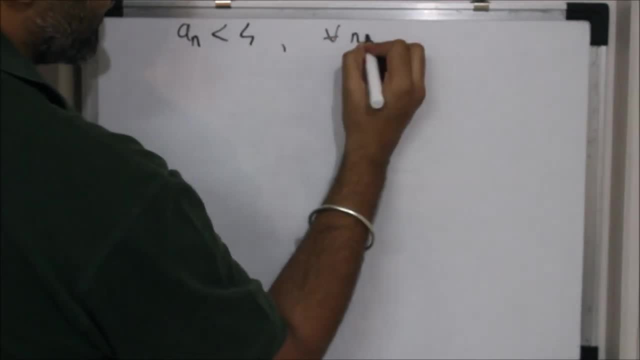 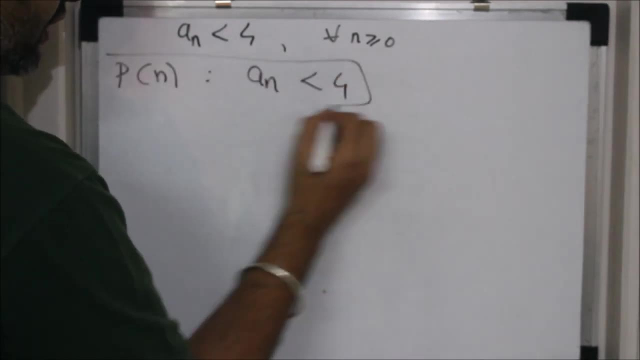 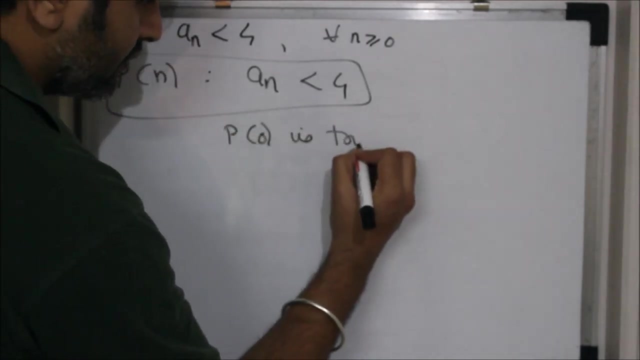 all the terms of the, an is less than 4 for all n greater, equal 0. so what is my p of n? my p of n is this statement: p of n is an is less than 4. again the proof by induction. now, what is our p of 0? is p of 0 true? yes, p of 0 is true. why? because your a naught is nothing. 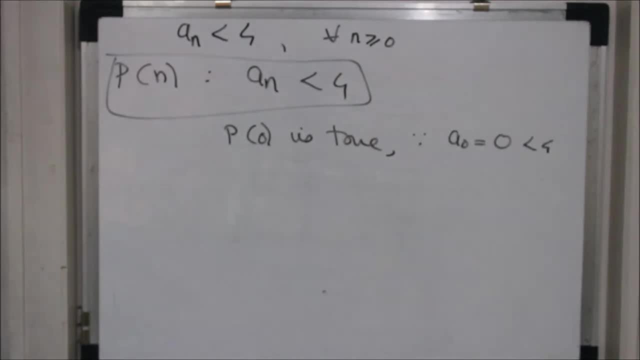 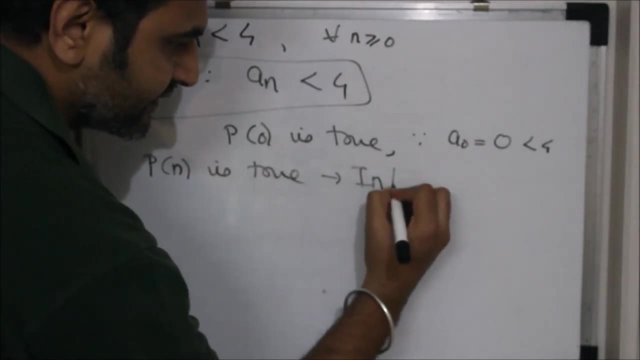 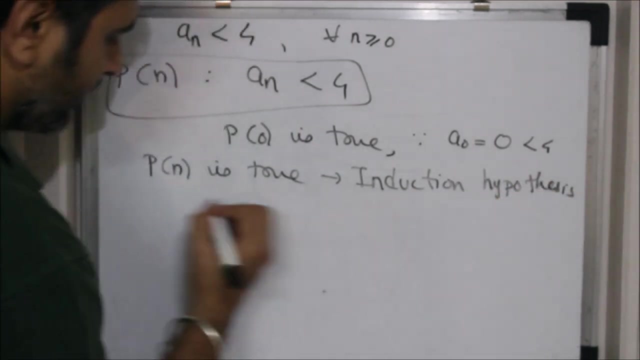 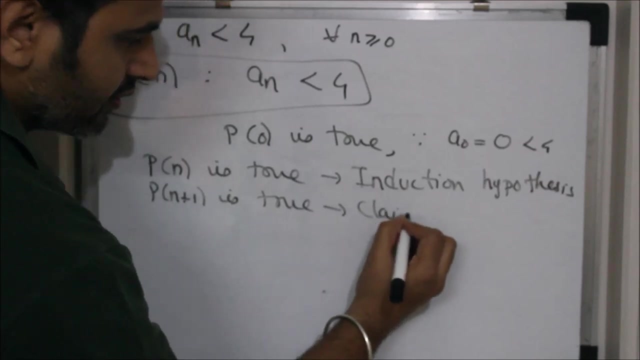 but 0, which is less than 4. so p of 0 is a true statement. now you assume that p of n is true. this is your induction hypothesis. and what is your claim? your claim is: p n plus 1 is true. this is your claim. so i want. 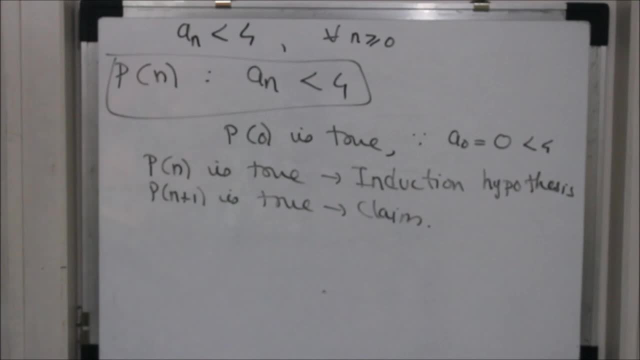 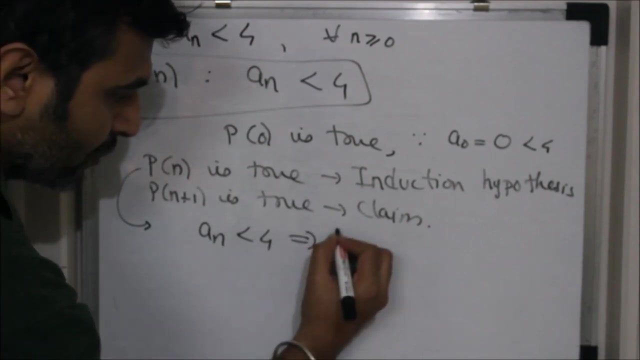 to prove this fact that p of n plus 1 is true. now, p of n is true means what this implies: your a n is less than 4, and what i want to prove? i want to prove that a n plus 1 is less than 4. so, using this fact, i will arrive at a n plus 1. so what to do is you multiply by: 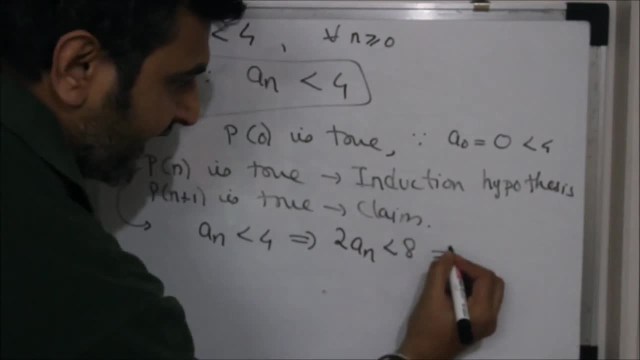 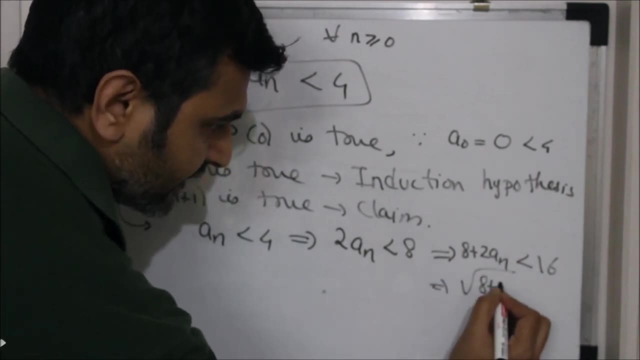 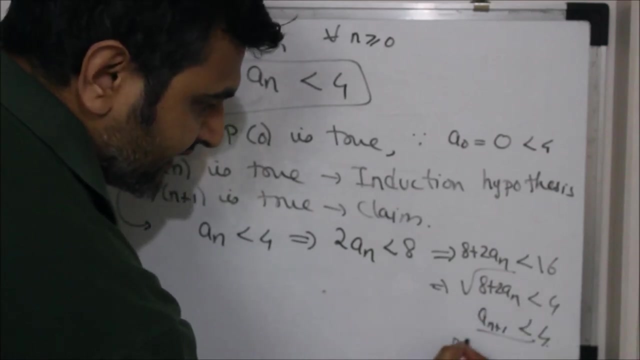 2 on both sides. you add 8 on both sides. 8 plus 2 a n less than 8 plus 8 is 16. you take square root on both sides. so 2 a n less than 4. but what is this? this is a n plus 1. so this implies what? 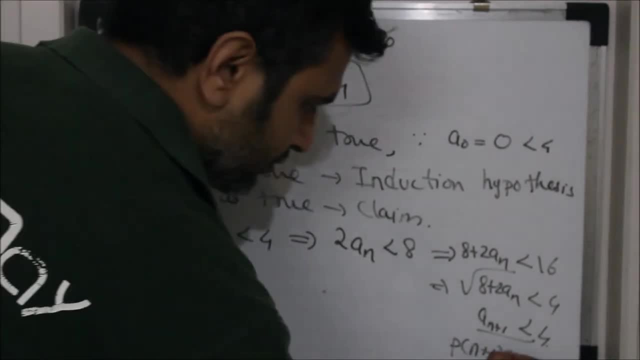 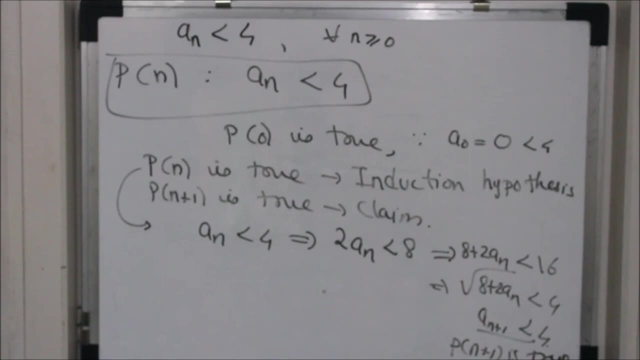 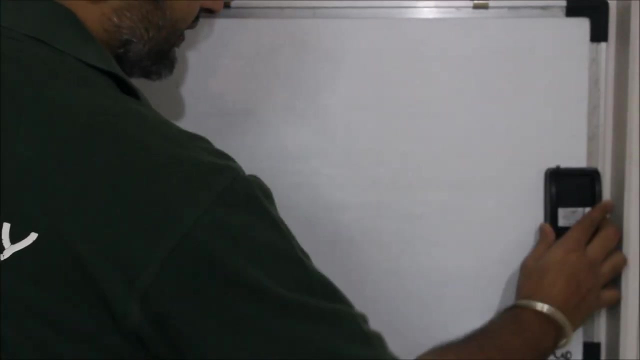 p of n plus 1 is true, so we assume that p of n is true and we proved that p of n plus 1 is true and therefore, by induction, n is true for all n. so therefore, what did we prove? is our sequence the recursive sequence? 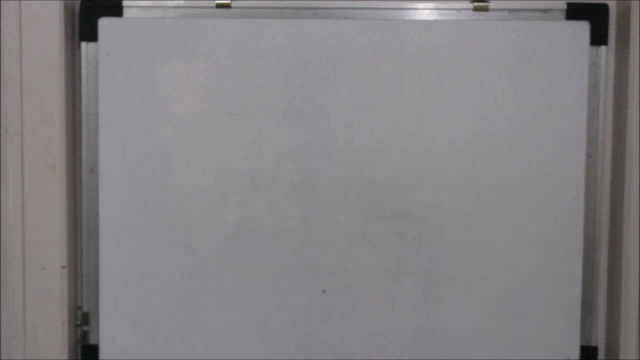 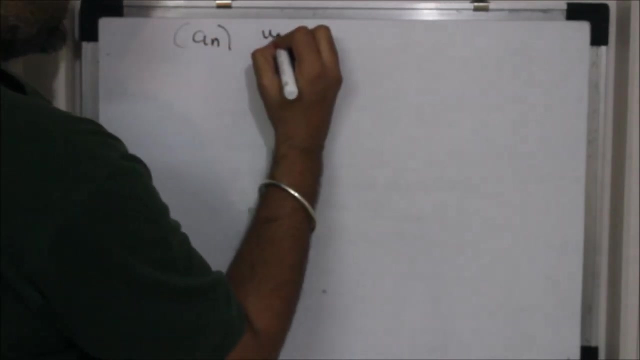 which we have is the increasing sequence and it's a bounded sequence. and therefore, by the theorem, by monotone bounded theorem, your a? n is a convergent sequence. and now, what is the limit? we know that zero, less than a n, less than four, is an increasing sequence. so 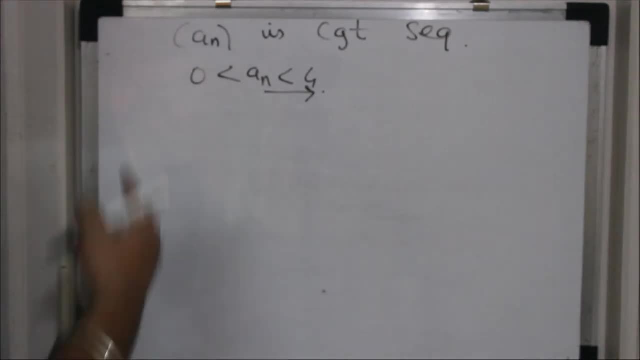 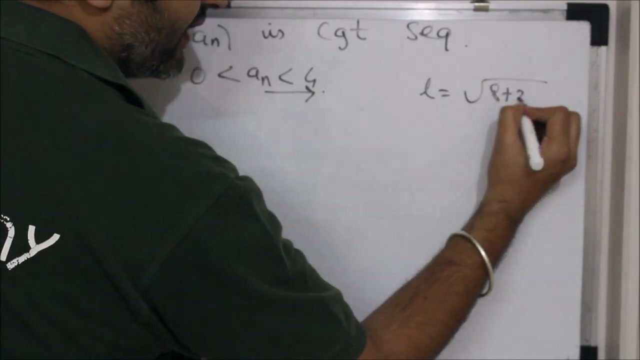 therefore it will converge to four. four is the limit of the sequence. and how do you prove? we just did a while ago. you assume l is the limit. so what you get l equal to root of eight plus two l, and by solving this we got l equal to four. so therefore the four is the limit. 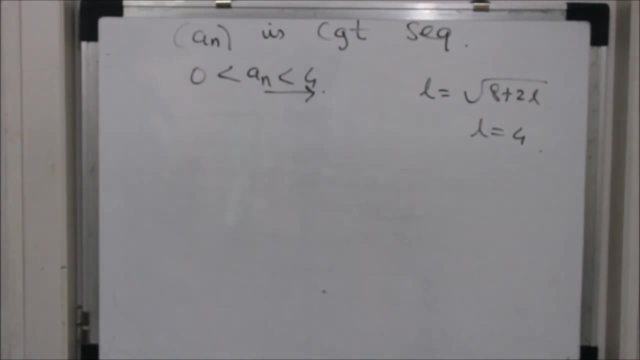 of the sequence. so this is how you solve a recursive problem. so you try to see whether it is increasing or decreasing by first writing few terms of the sequence and once you observe that fact, you try to prove that fact using induction. and here, since it was increasing, 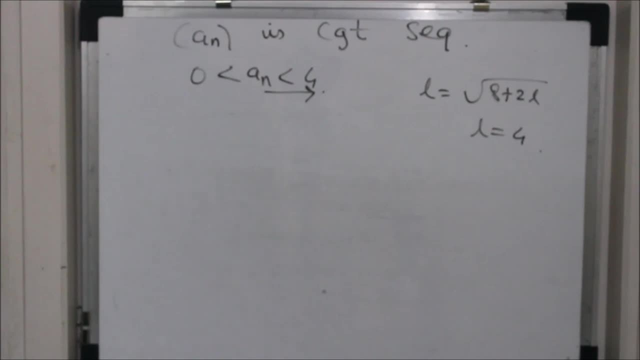 sequence. so we already have a lower bound, which is a one we wanted to find upper bound. so, using this trick, we found an upper bound and then we actually prove it. we actually proved that it's a upper bound. so that's how we prove that a recursive sequence is a convergent sequence. now I will give you one homework. 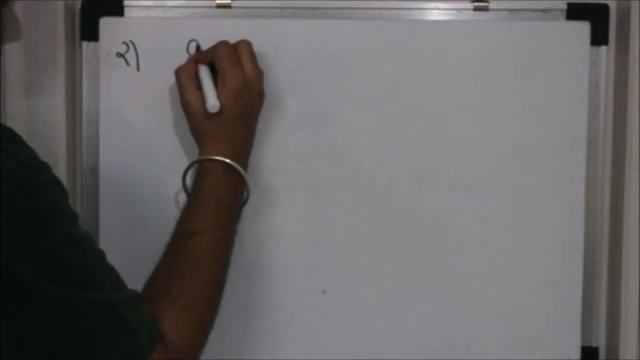 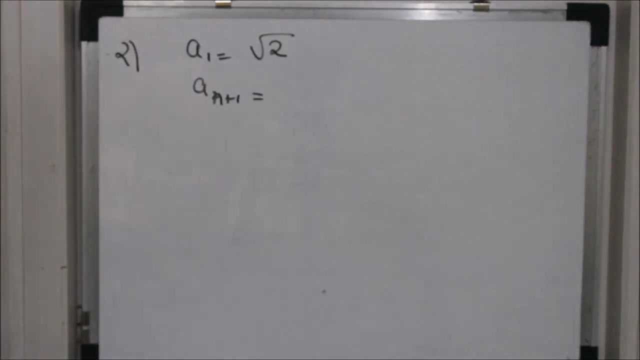 you try to prove that fact. so let a one be root two and a two and a n plus one be equal to root of two plus one. So let a one be root two and a two and a n plus one be equal to root of two plus one. 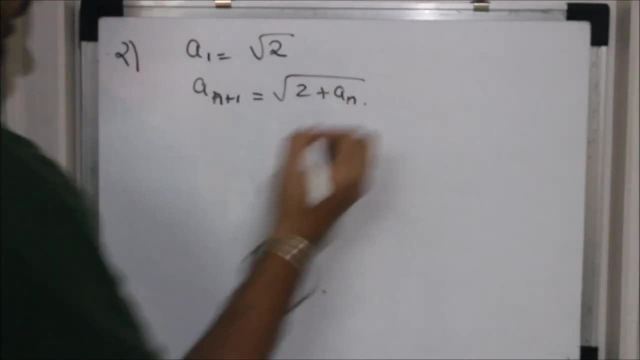 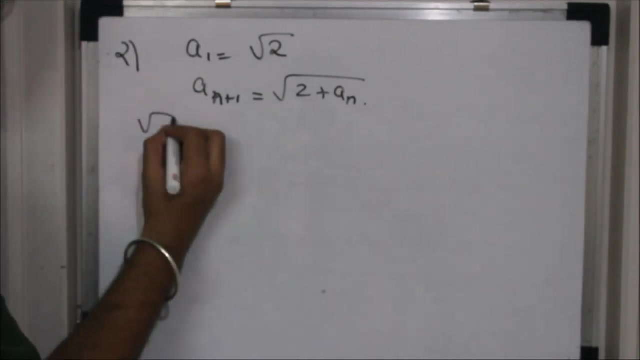 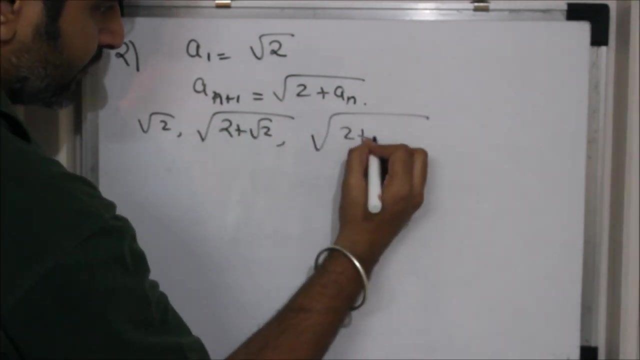 So here a one is root two. your a two will be root of two plus root two, and so on. so a one is root two. what will be a two? you put n equal to one, two plus a one. what will be a three? root of two plus root of two plus root two, and so this is a sequence and one. 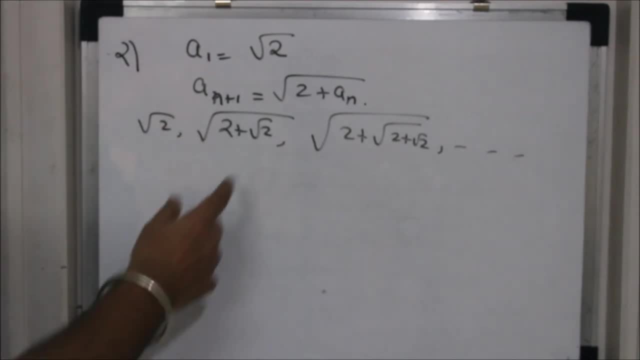 can say that this is an increasing sequence because I'm adding something positive, so I think this will increase. but then we try to prove this fact- it's an increasing sequence because a one is less than a two- and try to prove that a n is less equal a n plus one. 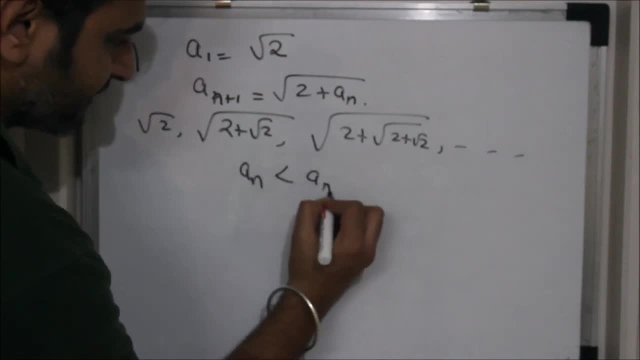 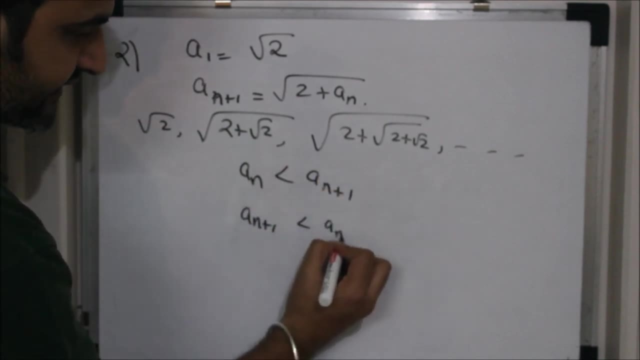 you assume the fact that a n is less than a n plus one. you add two on both side, you take square root on both side, and what you will get is a n plus one is less than a n plus two. so therefore, from there you can conclude that it's an increasing sequence. therefore, 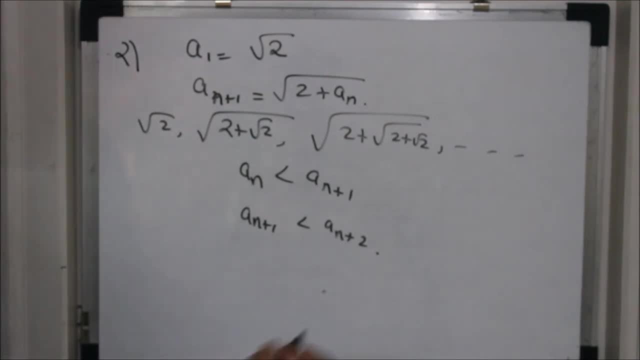 a one will act as a lower bound. a one will act as a lower bound. Question is: what is your upper bound? so you assume that this is a convergent sequence and it converges to l, so l equal to root of two plus l, and when you square on both side, 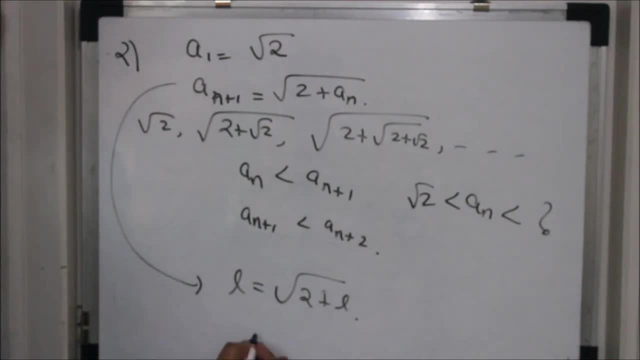 so when you square on both side, what you will get is you will see that your l is coming out to be two, and then you prove that all the terms of the sequence are less than two by induction. So idea is same, which I just did from for the previous question. 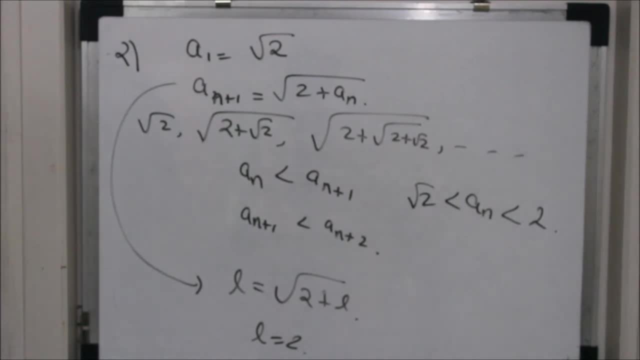 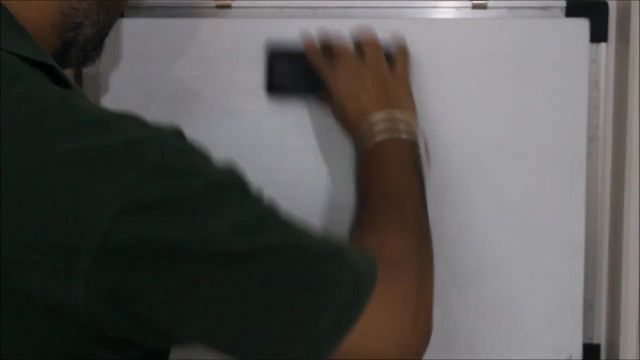 Same thing you have to do for the second question. So I gave you almost whole the hint. so you try to solve this problem. if you have any doubt you can ask me in the comment section. So this is the second example. let's go for the third example. 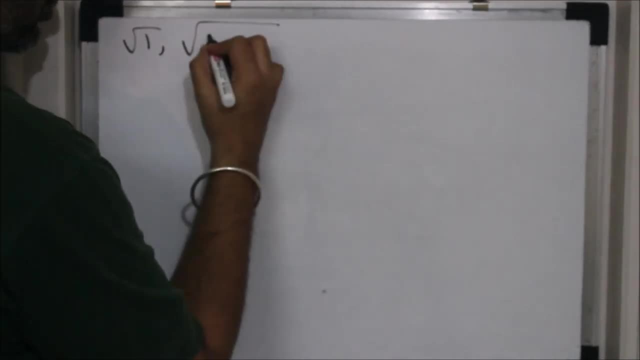 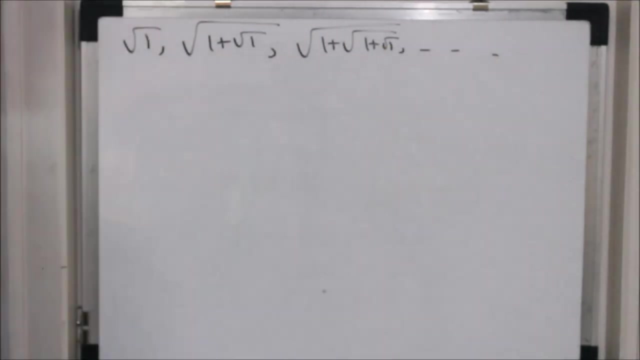 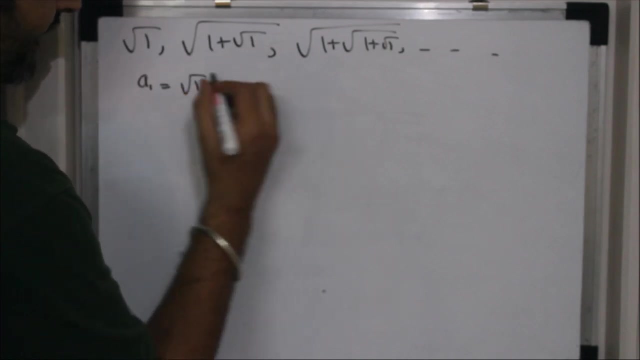 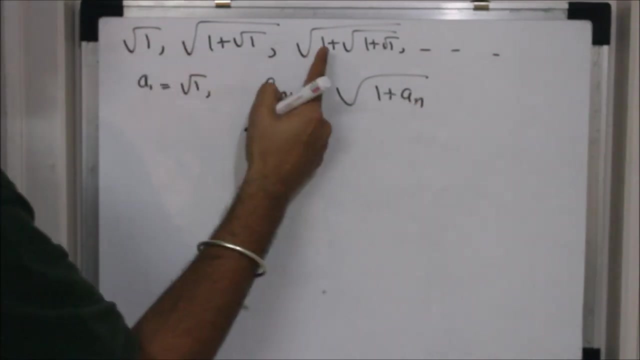 So suppose if I give you root one comma, root of one, plus root one comma, root of one plus root of one plus root of two, So what is my first term of the sequence? first term is root one and what is my a n plus one? it is root of one plus a n, one plus a one, one plus a two. so this is how I can construct. 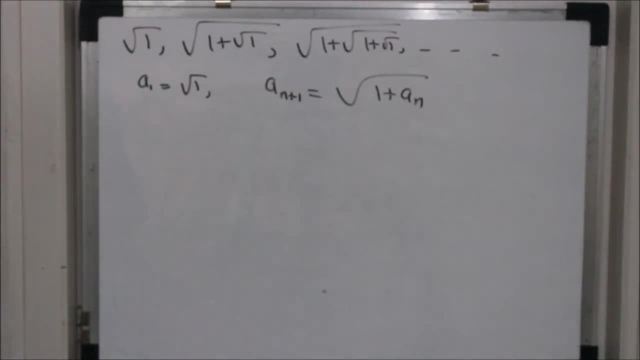 a formula for the recursive sequence. and now you have this recursive sequence again. do the same thing. one can see an increasing function. try to prove that a n is less than a n plus one. So this is an increasing sequence. so all the terms are bigger than a one. so root one is: 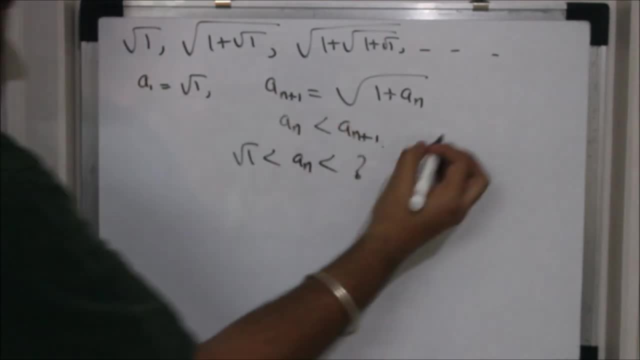 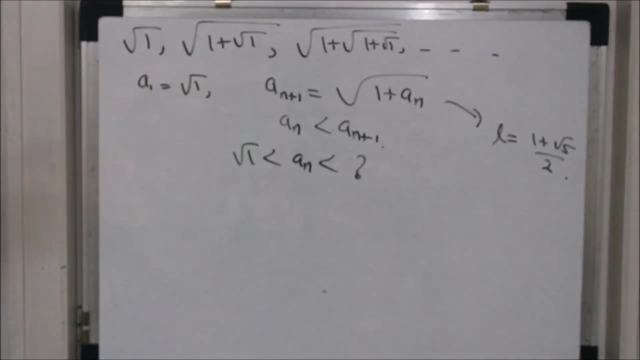 less than a n, less than what use the same fact. you will get l equal to one, plus root five by two. So that's what one has to prove. so again, this is an increasing sequence and it's a bounded sequence and therefore the upper bound. this will act as upper bound and therefore by bounded. 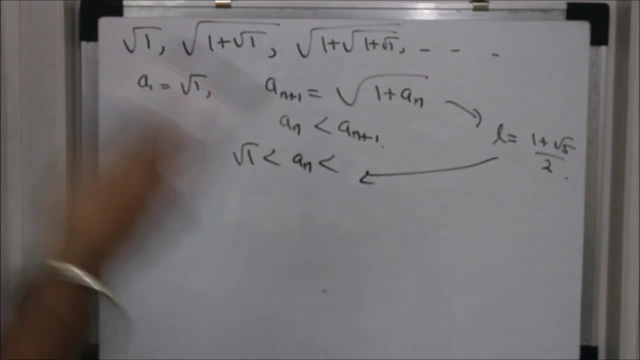 monotone theorem. this is a convergent sequence. Thank you Why I took this. it's the same example. there it was two, here this one. why I'm saying taking this? because this is a very nice number. if you have ever heard about golden ratio, that 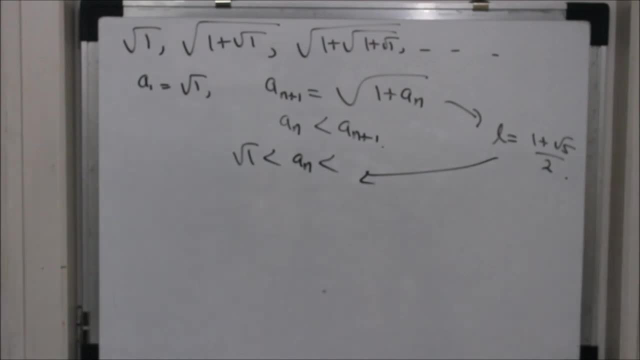 is a golden ratio. one can obtain using Fibonacci sequence. but yeah, this is a golden ratio used very widely or occur very widely. so this is one more example that sometimes a pattern will be given to you. from that pattern you have to derive a relation and then try to. 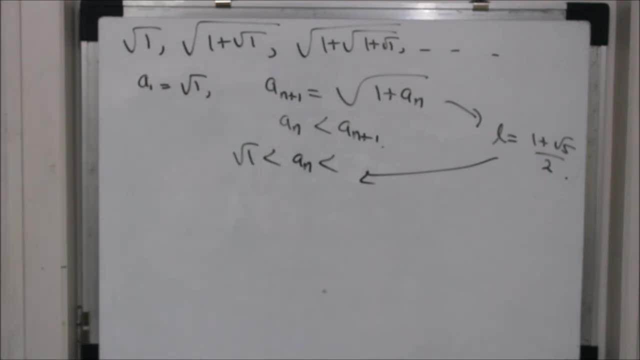 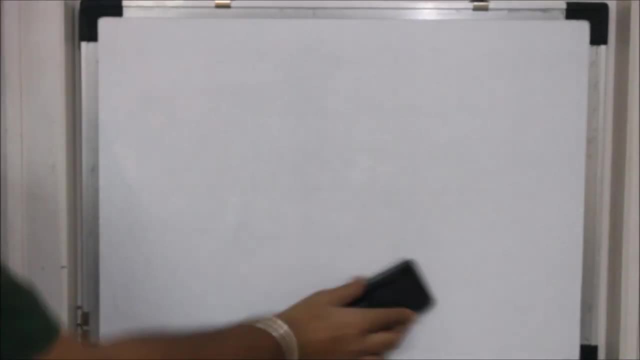 prove. it is monotone and it is bounded. So that's how you solve this problem. But every time induction may not help you. every time induction may not help you. So, for example, if I take another sequence, if I take fourth example, if I take a, one is: 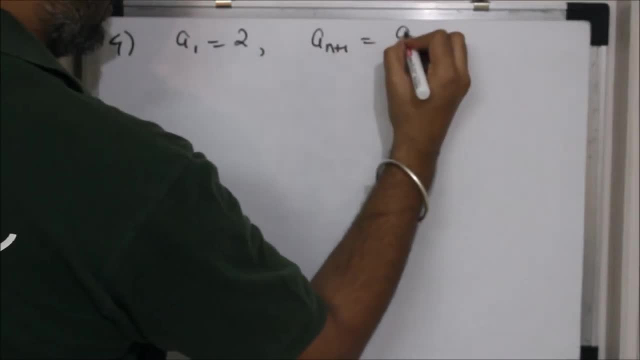 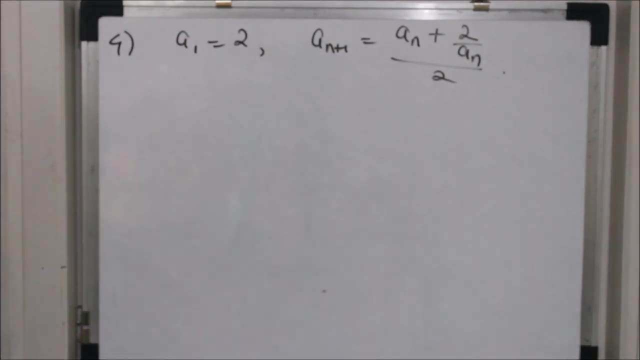 equal to two and a n plus one is equal to a n plus two upon a n. divided by two means one half of a n plus two upon a n. if I take this as a sequence, now I need to see whether this is increasing or decreasing. so if you try to write on few terms, it won't be that. 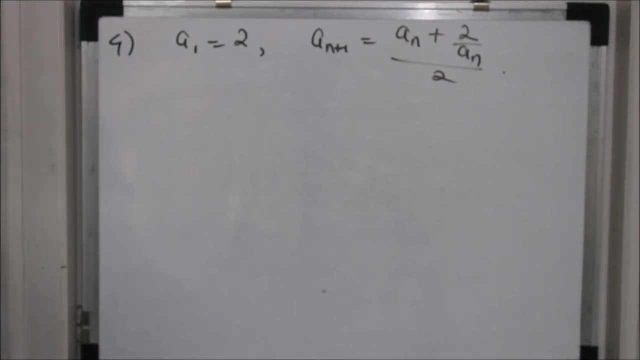 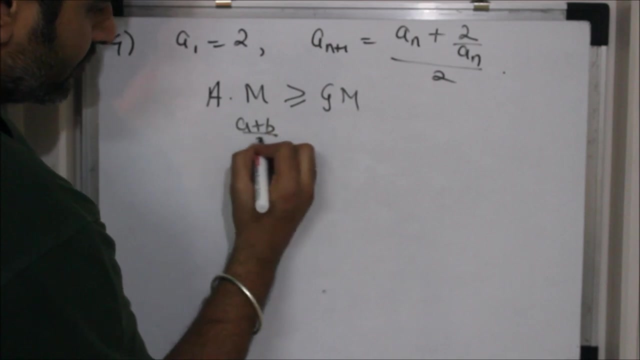 easy to prove. so here I'm going to use a trick. so you must have seen that arithmetic mean of numbers is always greater, equal. the geometric mean that means a plus b by two is greater, equal root of a, b. so if I take a as a, n and b as two by a, n, so what do I get? a, n plus two. 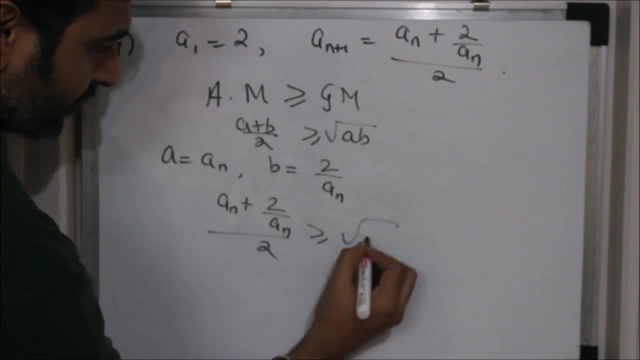 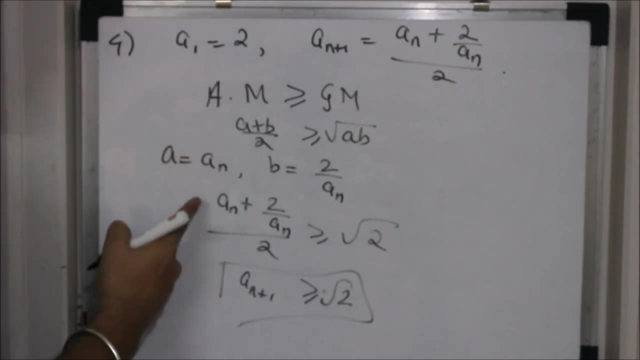 upon a n divided by two, greater, equal the product. what is the product? two and what is this? this is my a n plus one and this is true for any n right if I take a n equal to one, so a one plus two upon a one by two greater, equal root: two: a two plus two upon a two greater. 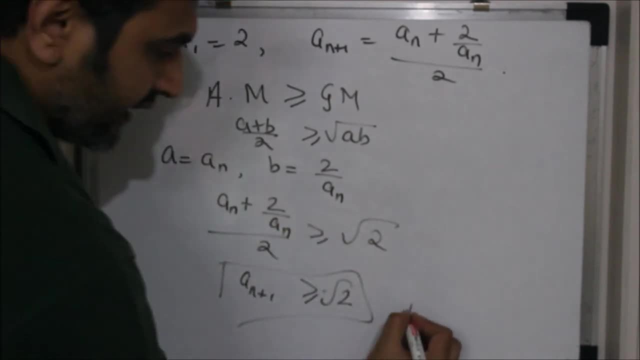 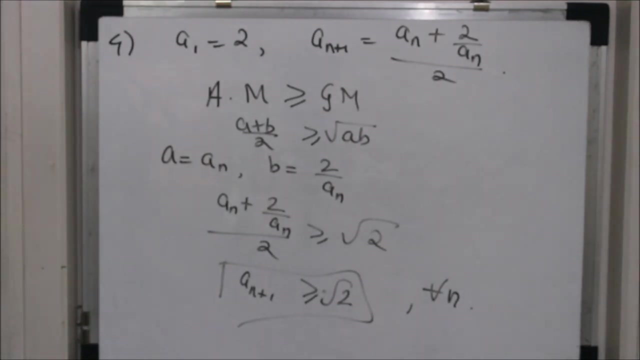 equal root two, a three plus two by a three upon two, greater equal root three. in short, this is true for all n. so what I get is- I'm getting a lower bound for this sequence- that n plus one is greater equal root two. so I got the lower bound for the sequence now question: 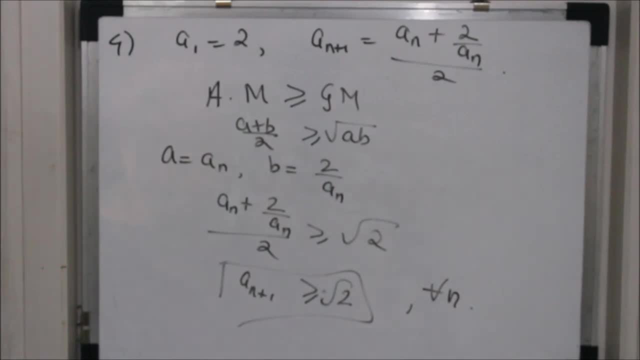 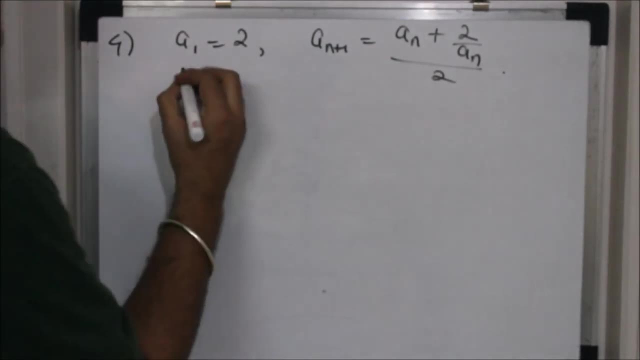 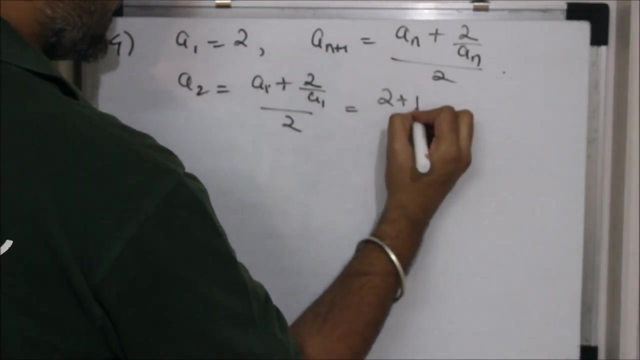 is what is the upper bound of this sequence? so if you observe, if you observe over here, my a one is two. what is our a two? what will be our a two? it will be a one plus two upon a one upon two, so it is two plus one by two, which is one point five. so what you are getting, 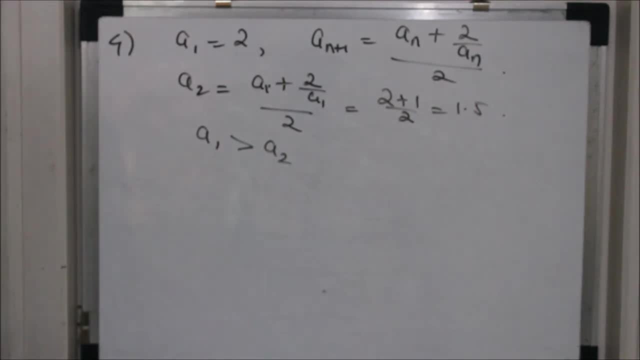 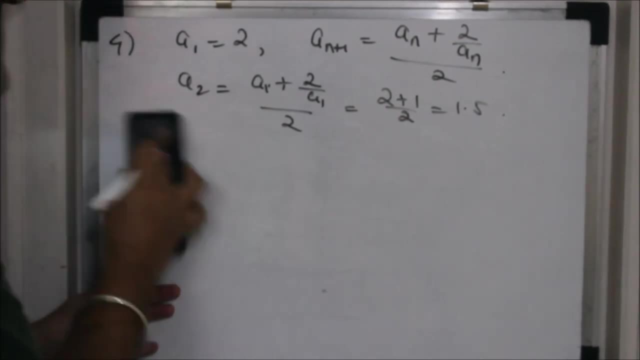 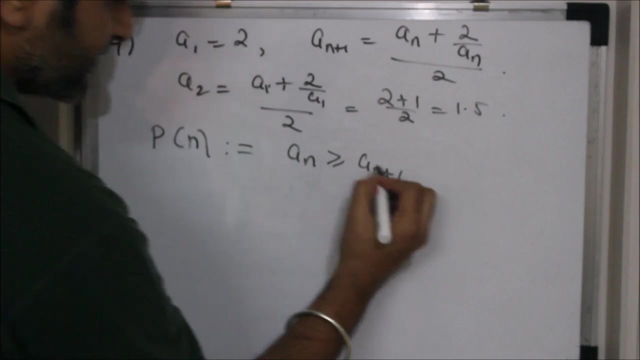 a one is greater than a two. so in this case, one can see that it's a decreasing sequence. so let's try to prove this. so let's try to prove that this is a decreasing sequence. so what is my statement? my p of n is a. n is greater, equal a n plus one. this is what I want to. 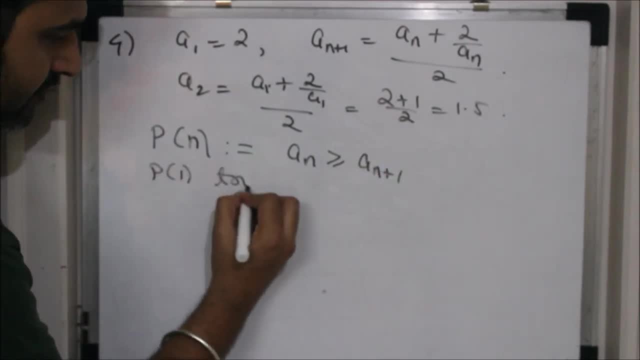 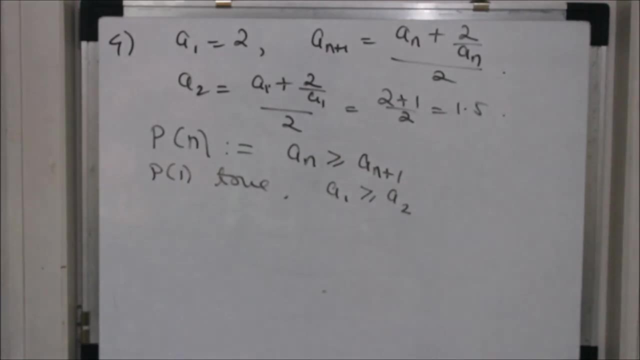 prove p of one is true because your a one is greater, equal a two. one can see this is true. this is one point five. so a one is greater than a two. therefore, p of one is greater than a two. therefore, p of one is true because your a one is greater, equal a two. one can see this. 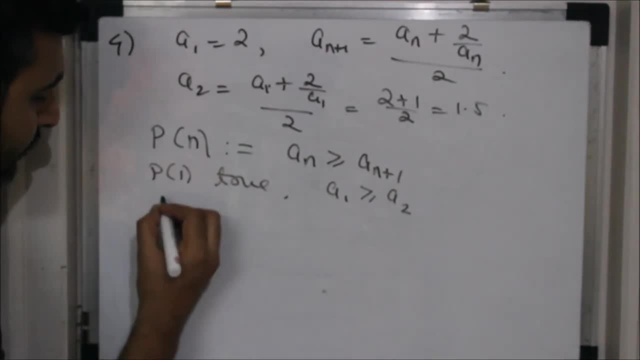 is true. this is one point five. so a one is greater than a two. therefore, p of one is greater than a two. therefore, p of one is greater than a two. therefore, p of one is greater than a two. 2. now assume so now what I want to prove, that I want to prove P of n is true, or? 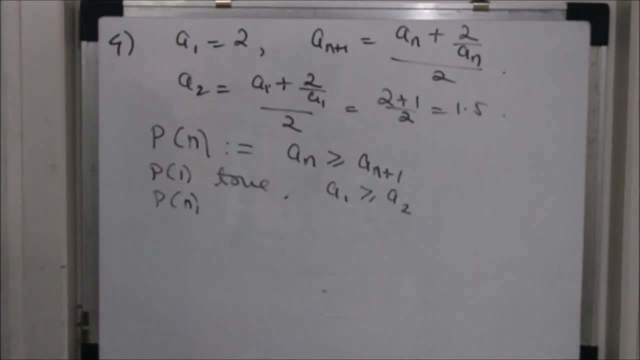 you assume P of n is true and you prove that P of n plus 1 is true. that is one way of doing that, but I won't go by that. I won't apply induction over here. why? because I mean, you can try over this, that's not a problem. but what I want to 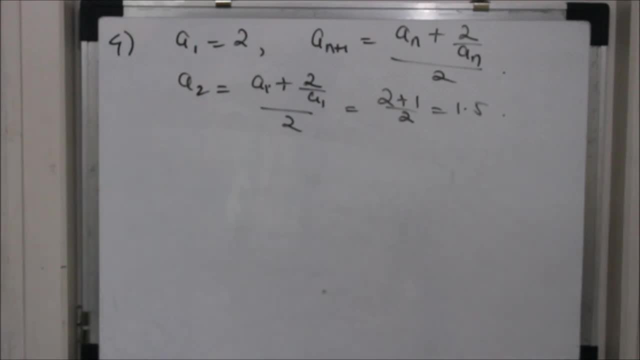 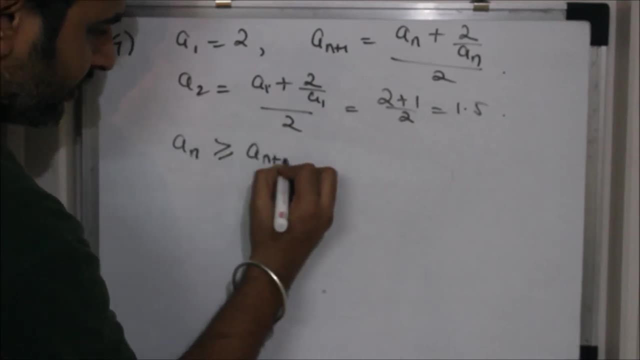 say, is sometimes, even without induction, you can prove. there's something, I mean a statement, is true. now, what I want to prove over here is: a n is greater, equal a n plus 1 for all n. right. see, induction is a tool which will help you always, but 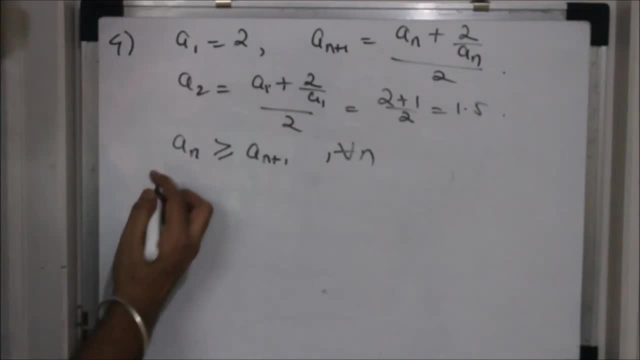 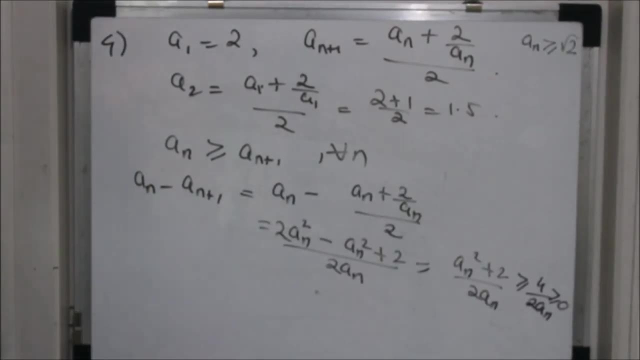 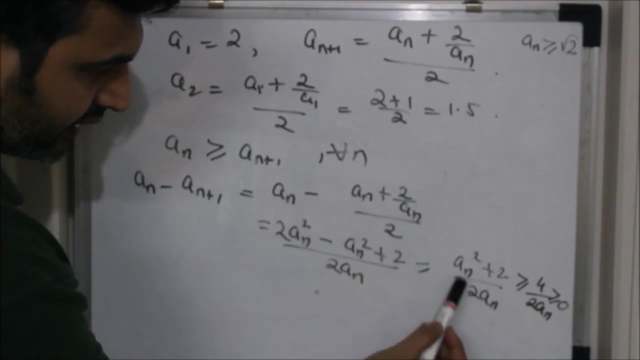 sometimes also need to apply some ticks. so here what I want to prove: that a n minus a n plus 1 is greater equals 0. so what do we get is a n minus a n plus 1, is a n upon a n plus 1. if I do this adjustment over here, what I get is a n. 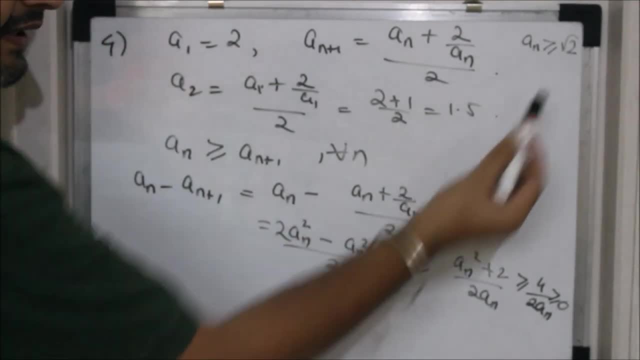 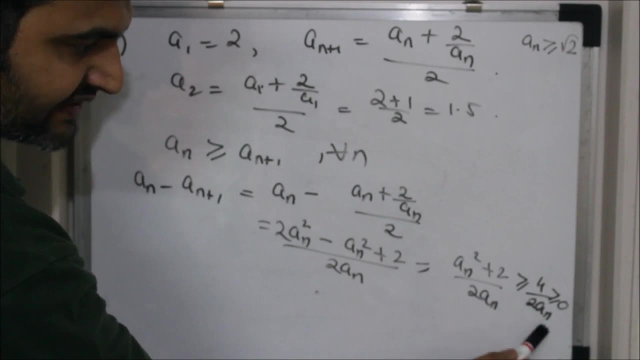 square plus 2 upon twice a n. but we just saw that a n is greater, equal root 2. so if I square it I get 2. so a n square is greater than 2. so 2 plus 2 is 4 upon twice a n. so since a n's are positive, 4 upon twice a n is positive. so what do I? 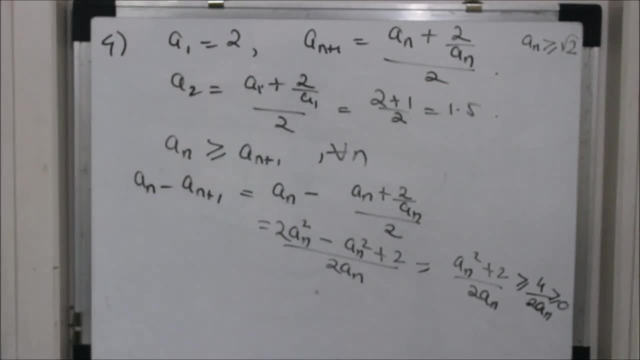 get is a n minus a n plus 1 is a positive number and therefore what do I get? is a n is greater, equal a n plus 1 for all n. so here one can try by induction, or if you feel that induction is a difficult thing, one can try. of this different, different. 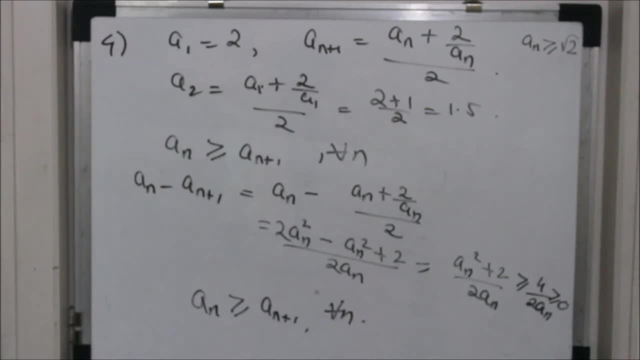 techniques. so for lower bound, I use am-gm inequality, and for decreasing, to show that the sequence is a decreasing sequence, I use the fact that I need to prove that the subtraction is greater equals 0. so this is one more trick, one which can use if you are facing difficulty in induction. so what do we? 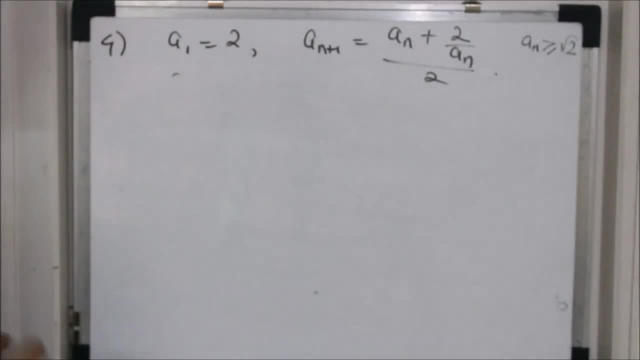 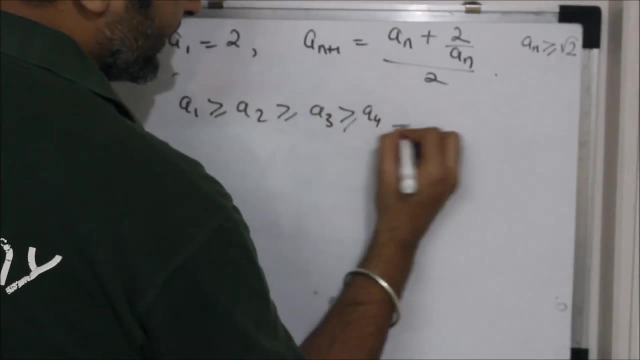 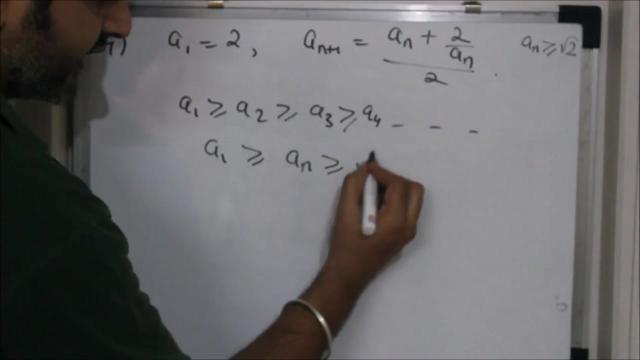 have proved. what we proved for this sequence is that it's a decreasing sequence, means a 1 greater equal a 2 greater equal, a 3 greater than a 4, and so on. so it's a decreasing sequence. so what is the upper bound? a 1 is the upper bound and we know that root 2 is the lower. 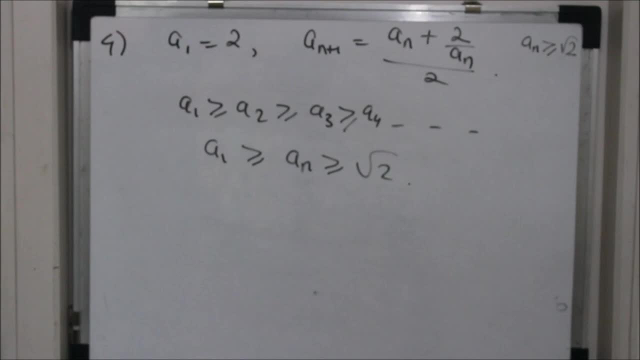 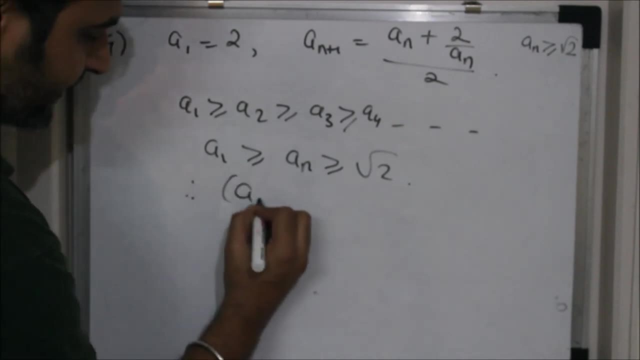 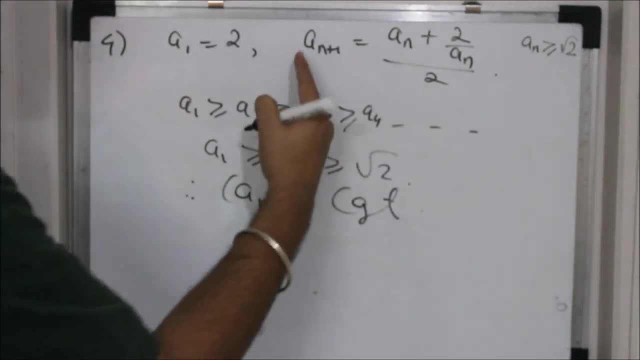 bound for the sequence, because we just now proved that all the terms are greater, equal root 2. so therefore your a? n is a bounded sequence. also, it's a monotone sequence. therefore, your a? n is a convergent sequence and using the same trick. so if this is converging to L. 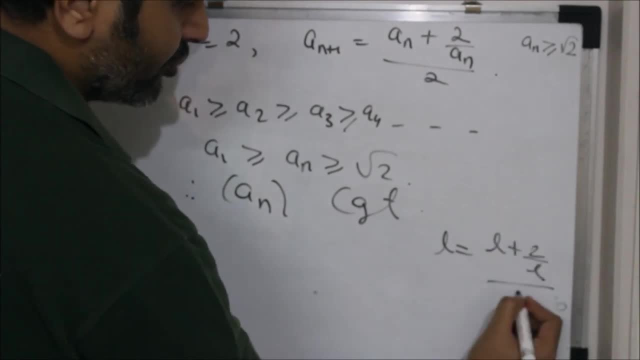 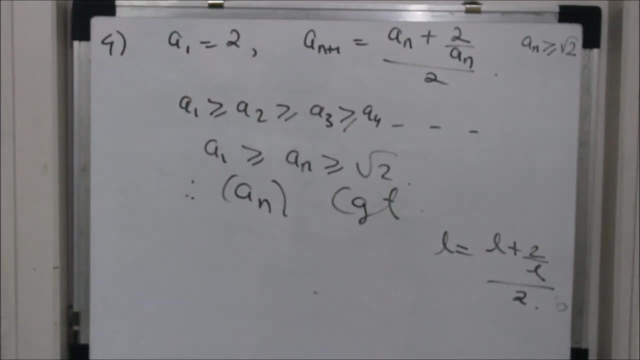 L equal to L plus 2 upon L upon 2. you try to solve this. what you will get is you get L equal to root 2. so therefore, root 2 is the limit of this sequence. so this is one way of solving this kind of problem. and let's take one last example. 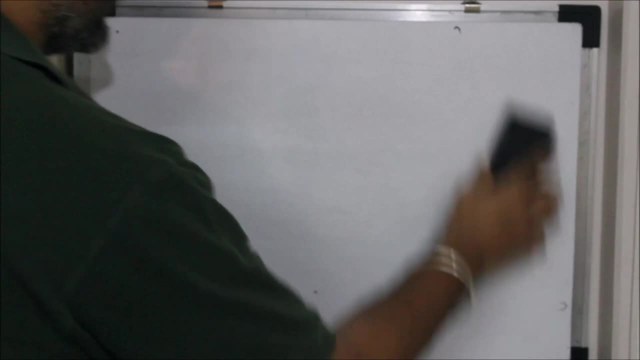 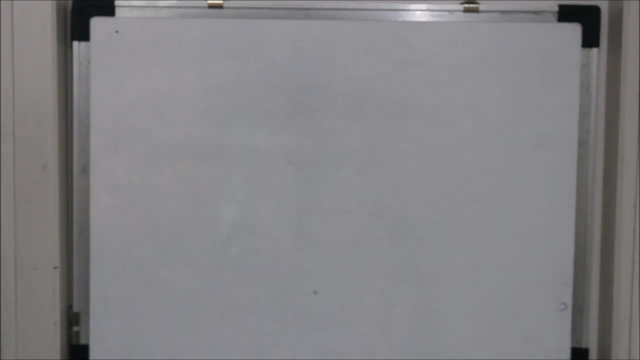 let's take one last example. so, like in the first previous problems I took the help of induction. in this problem I used took help of some tricks like am-gm and that subtraction is positive. one more trick: what you can do is if I give you another sequence, suppose if I take a 1 equal to 1 and a n plus 1 is a n plus 1. 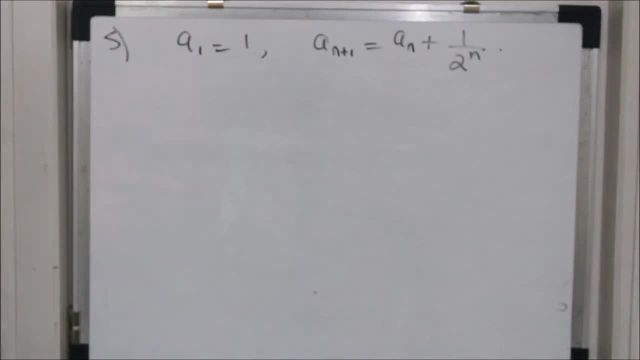 upon 2, raised to n. now I want to show that this sequence is a convergent sequence. so now let's see whether this is increasing or decreasing. one can clearly see that I am adding one, some positive number to a n to get a n plus 1. 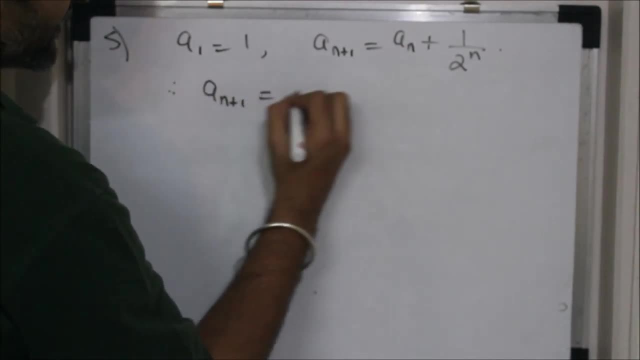 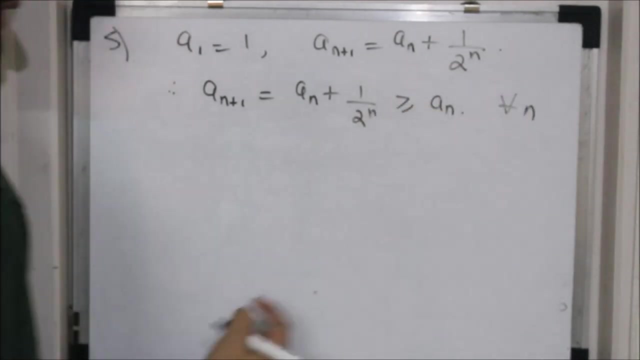 so from here I can see that your a n plus 1, which is nothing but a n plus 1 upon 2, raised to n. this is what greater equal a n. this is true for all n right, because for all n I am adding something positive. so what do I have? a n plus 1 is. 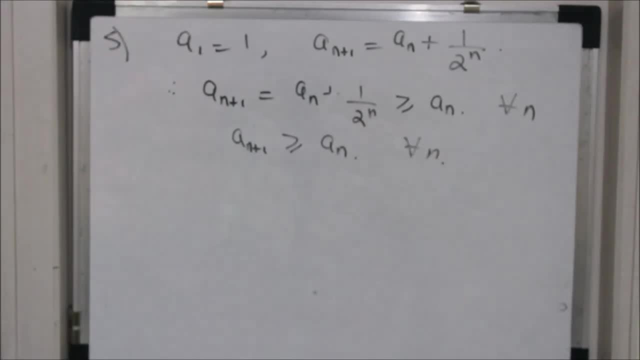 greater equal a n for all n. so therefore this is an increasing sequence. so without even induction, I can prove that this is an increasing sequence. so now this means what I have: a 1 less equal a 2 less equal a 3. this is what I have. so now I want to show n. a 1 is acting as a lower bound. 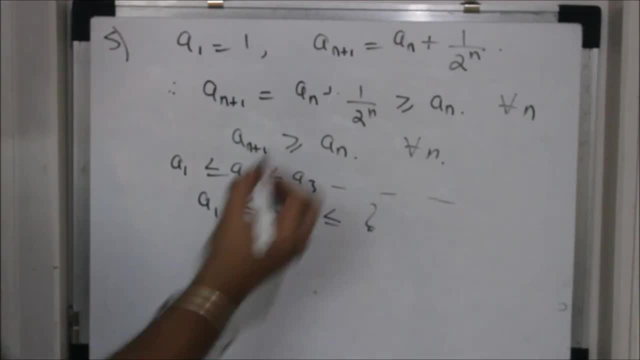 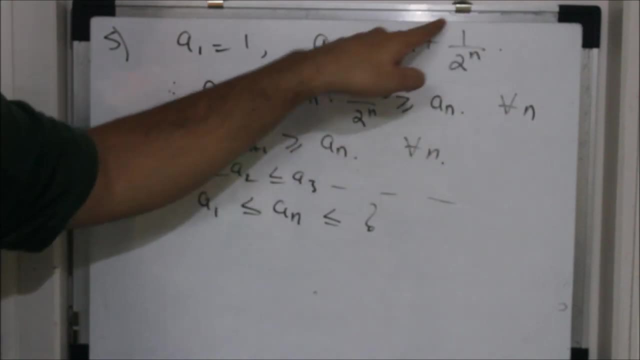 question is: what is the upper bound? now here I cannot apply the previous trick that suppose this is converging to L. what I'll get- L equal to L plus this goes to 0- is a sequence, so I get L equal to it. so that trick is not helpful over. 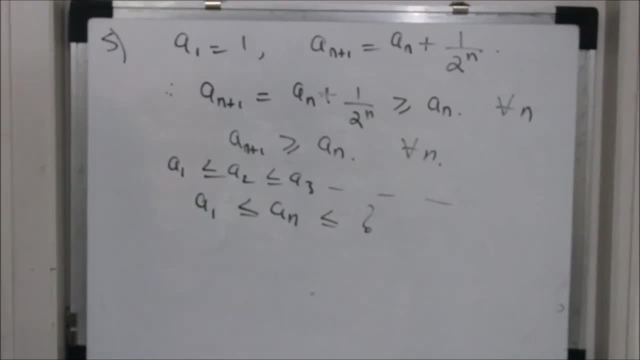 here to what is to find the limit of a sequence. so what we'll do is we will try to write down the terms of the sequence. see what my aim is. I prove it is monotone. I got the lower bound, I wanted the upper bound, so I want the upper bound for the sequence. so what you do is: 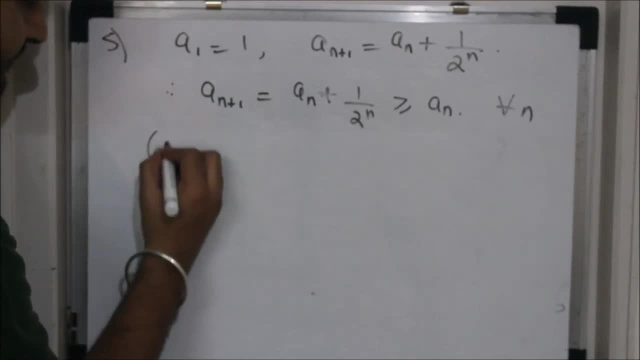 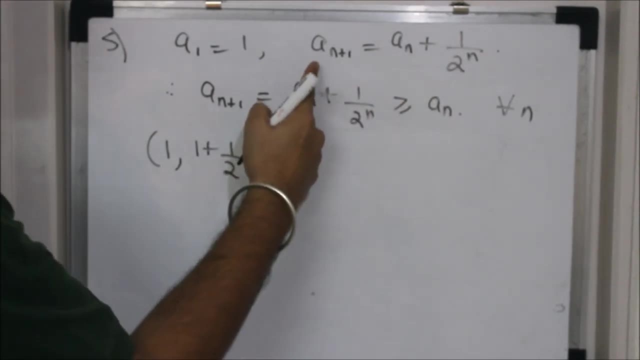 you try to write down the terms of the sequence, so my first term is 1. what is a 2? you put n equal to 1. a 1 plus 1 by 2. 1 plus 1 by 2. what is a 3? you put n equal. 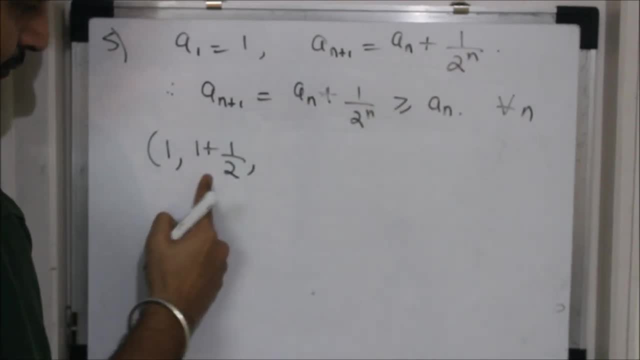 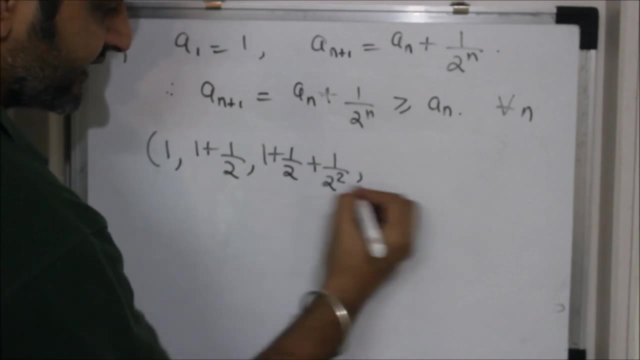 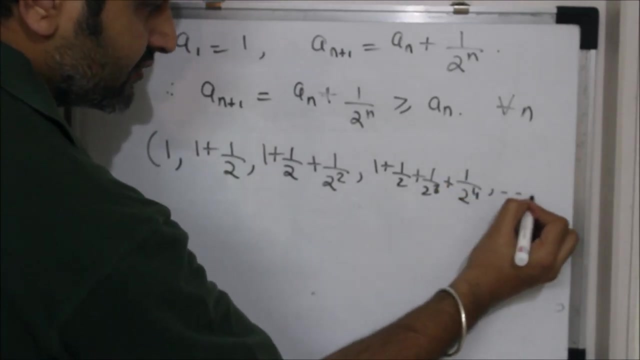 to 2. a 2 plus 1 by 2 square. a 2 plus a 2 plus 1 by 2 square. what is a 4? it will be. a 3 plus means a 3 plus 1 upon 2 raise to 4 and so on. so if you, 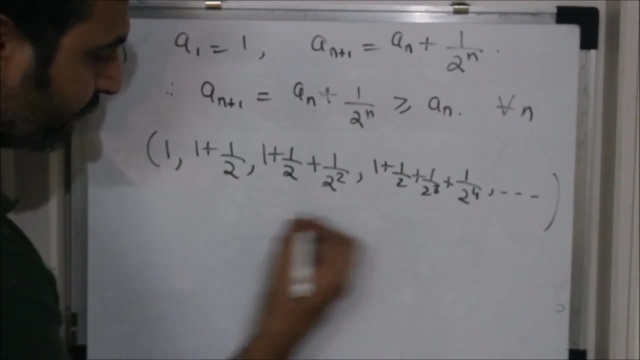 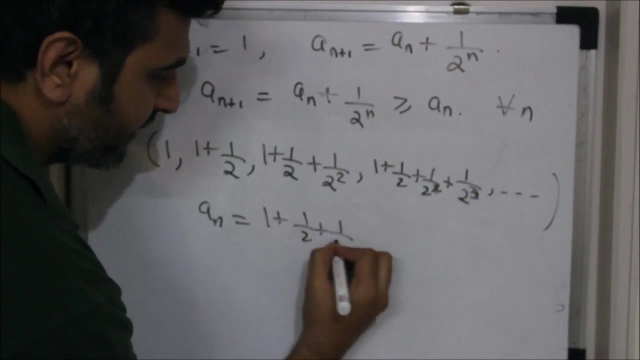 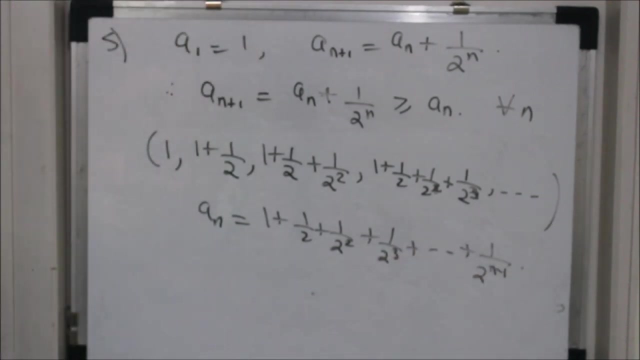 observe your a: 1, a 2, a 3, a 4. in general your a? n is nothing but 1 plus 1 by 2, plus 1 by 2 square plus 1 by 2 cube plus 1 upon 2 raise to n minus 1. so this is: 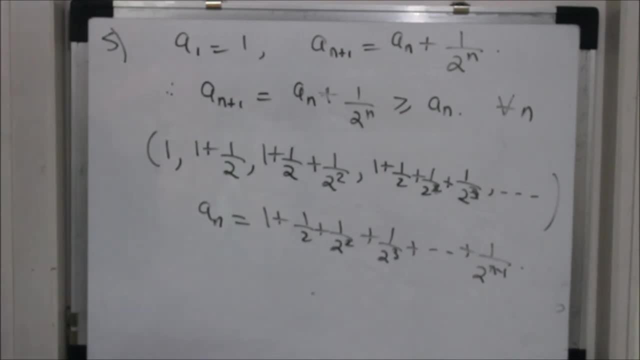 what that a, n is. and now, as n goes to infinity, you know that this is a geometric series. if you have any doubt in the geometric series, you can see my lecture on geometric series in the playlist of series of real numbers. but then here, since as n goes to infinity, this is: 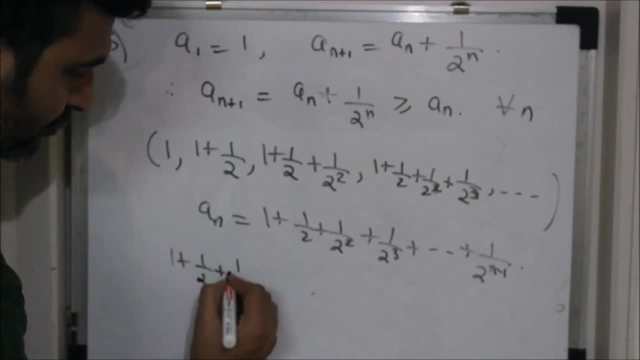 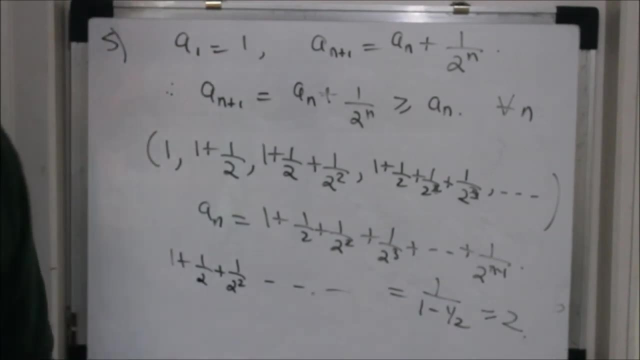 nothing but a geometric series and 1 plus 1 by 2 plus 1 by 2 square. this converges to 1 upon 1 minus half, because common ratio is half. so this is converging to 2. that means what all a n's are less than 2. why? because what is a n? 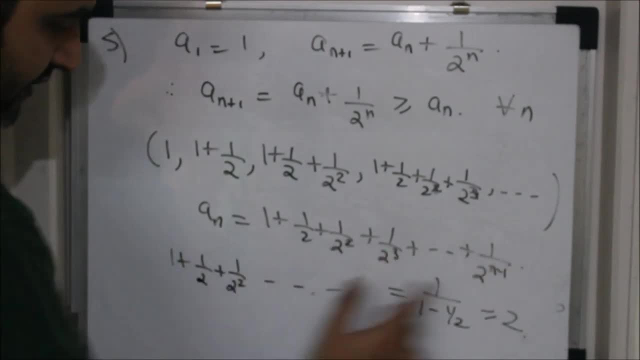 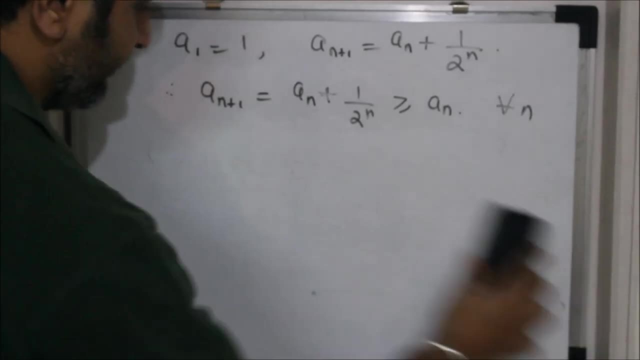 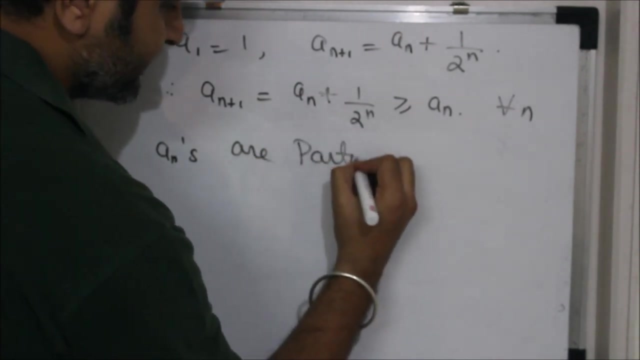 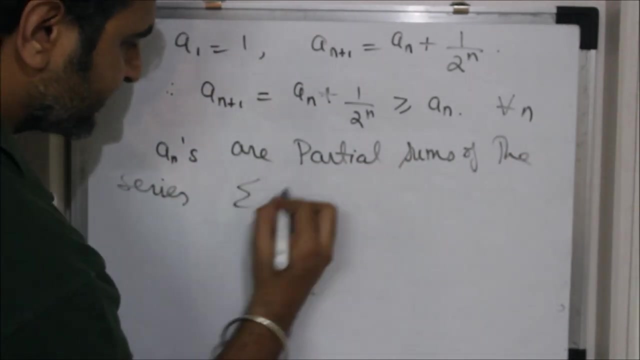 I am taking the partial sum of this series and obviously all infinite sum is giving me 2, and this is the partial sum. so what you can say is what you can say is your a- n's are partial sums of the series. summation 1 upon 2 raise to n, which is nothing.